This is basically the ideal composition which we should have. So for the next 50% of the soil volume it should be pore space and out of this 50%, 35% should be soil air and less 35% should be soil water. 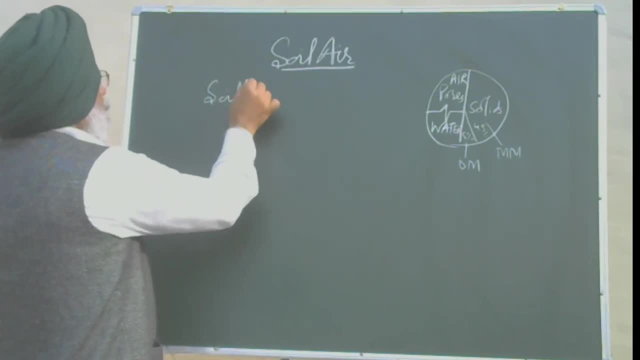 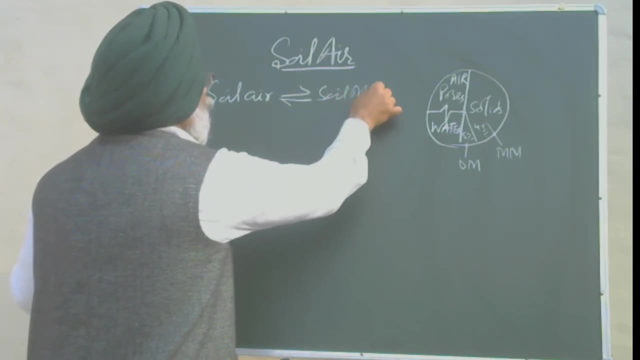 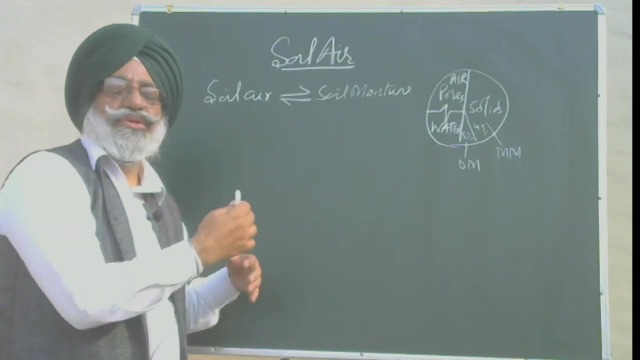 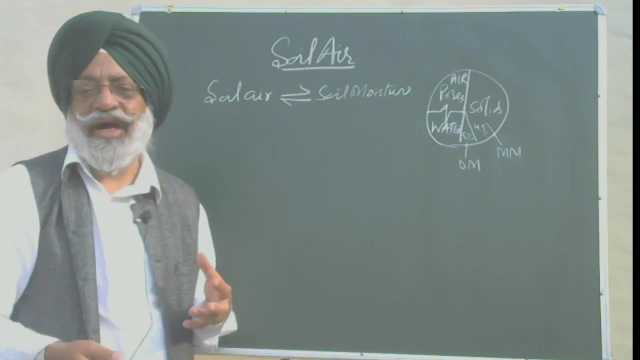 So that means soil air and soil water or soil matter For soil moisture. you can see these are interdependent. If you have higher amount of soil moisture, soil air content will be low. On the other hand, if you have lower amount of soil moisture, soil air content will be high. 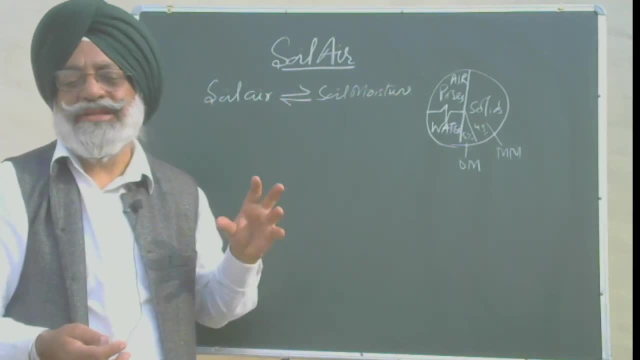 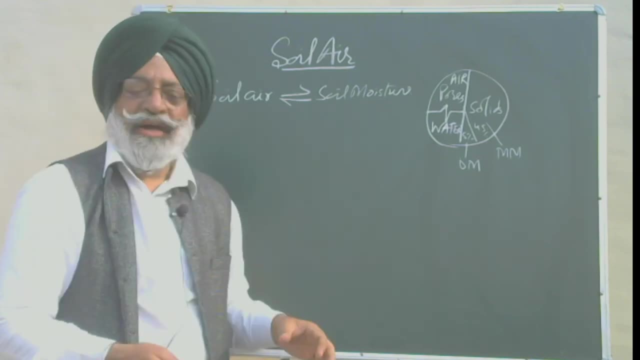 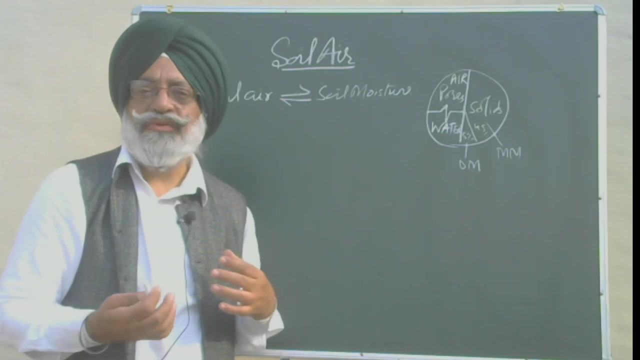 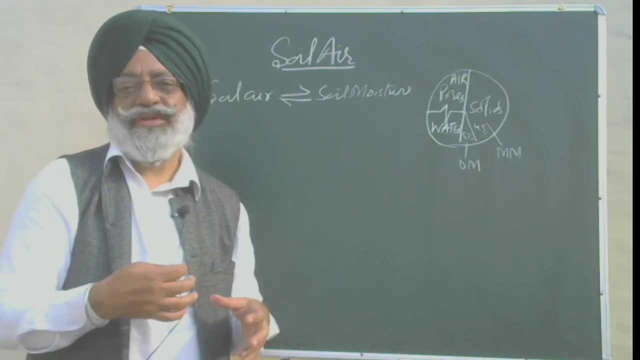 Now the question is why we should have a proper balance of water and air in the soil. It is because the plant roots need water for meeting its transpiration activities, For uptake of nutrients in solution form. At the same time, the plant roots also need oxygen to breathe, except, you know, the aquatic plants. But since we are concerned with agriculture, so I should say, except rice plant, all other crop plants- they have the mechanism of plant roots breathing independently of the aerial parts from the soil. So that means plant roots, they need oxygen to respire in the soil and they, of course, they take up oxygen and they release carbon dioxide as every living being does. 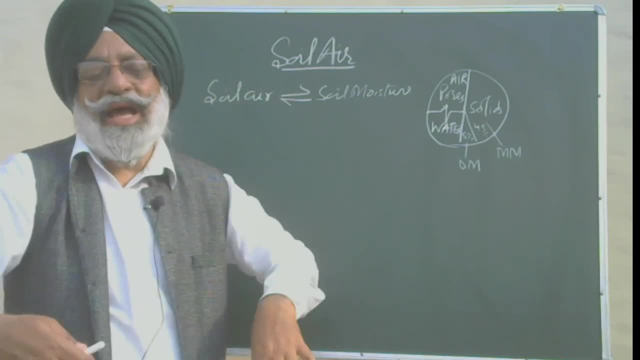 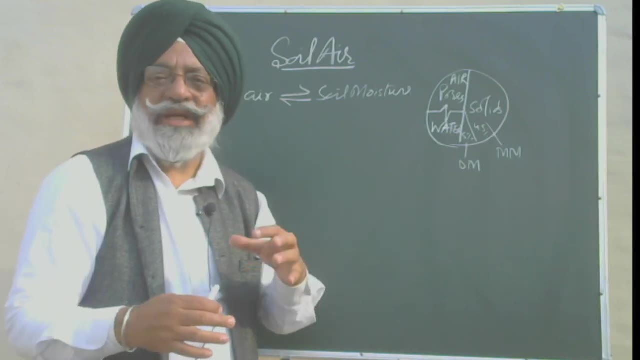 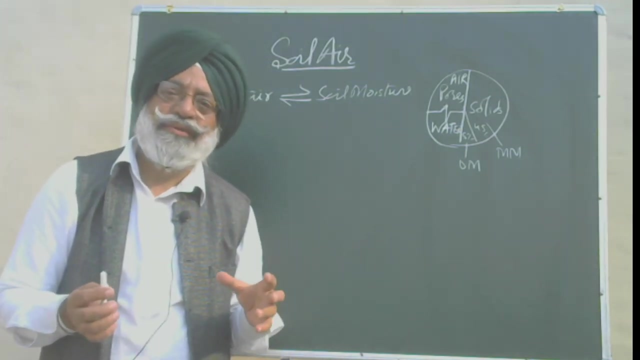 Like human beings, we take up oxygen and then give out carbon dioxide. Same is true with the plant roots. So it's very important to maintain a balance between soil moisture and soil air. If you remember, in my introductory lecture, I told you that why soil physics is important. 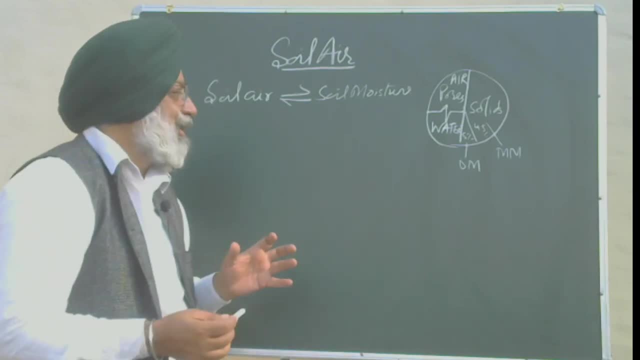 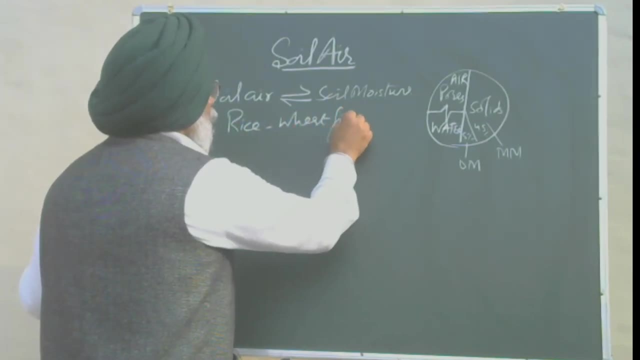 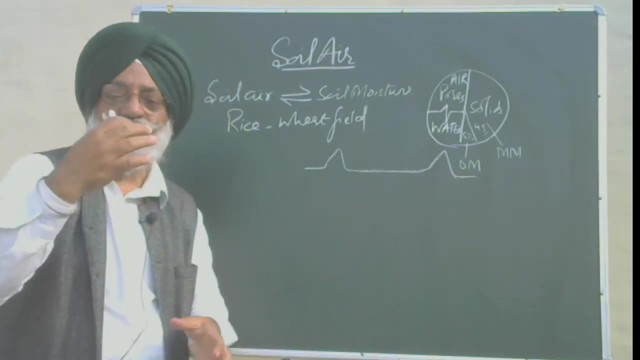 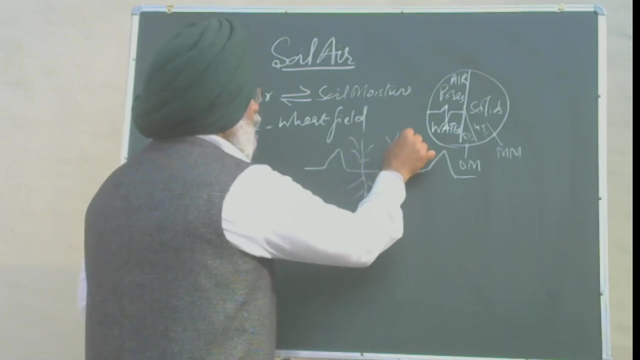 So here I will again give an example, that if you have a rice-wheat field, For example, say if this is a rice-wheat field. So you know, in rice we go for continuous puddling And then after rice you go for wheat crop. 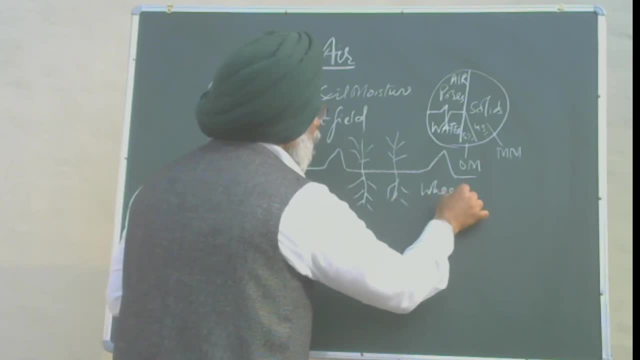 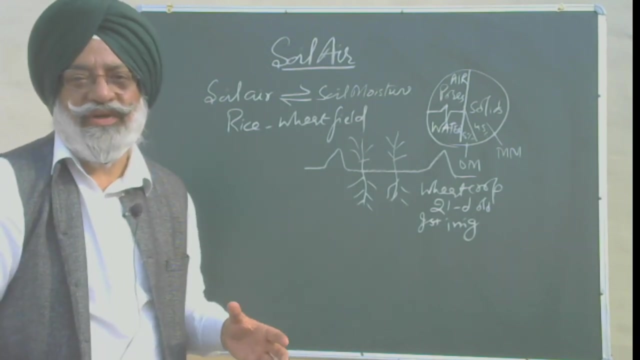 So wheat crop is. So wheat crop is in the field and it is 21 days old crop. So when we go for first irrigation, So coincidentally, when you have irrigated the field, either you give a heavy irrigation or, if it's a normal irrigation plus rains occur. 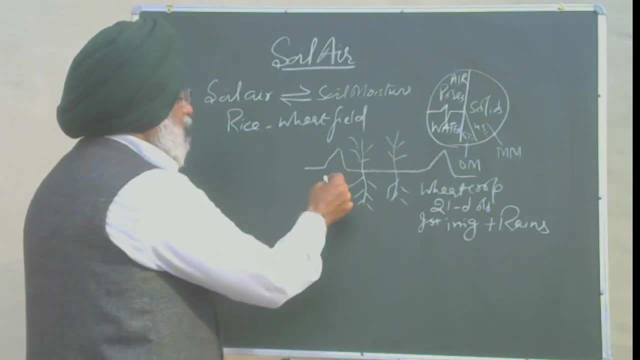 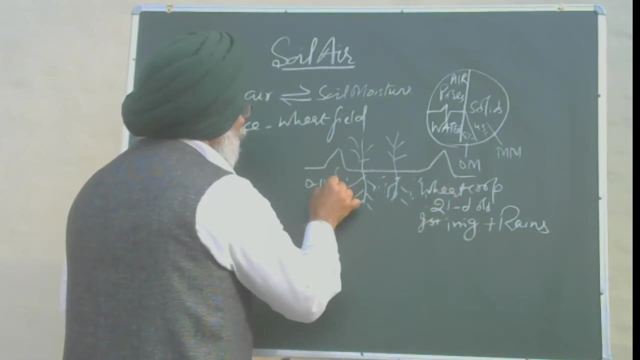 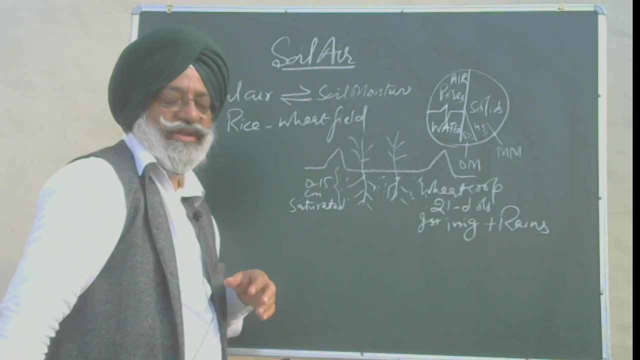 So in that case there will be temporary water logging conditions in the soil And this 0 to 15 centimeter zone. this will become saturated, more or less saturated. So when we say saturated means almost whole of the pore space is filled by soil moisture. So ultimately the roots also. if it's a 21 or 25 or 28 days old crop, the roots are just within 0 to 15 centimeter. So if all the pores are filled with water, obviously there will not be any air. 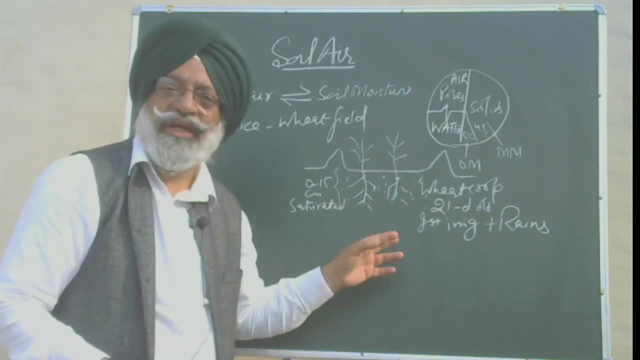 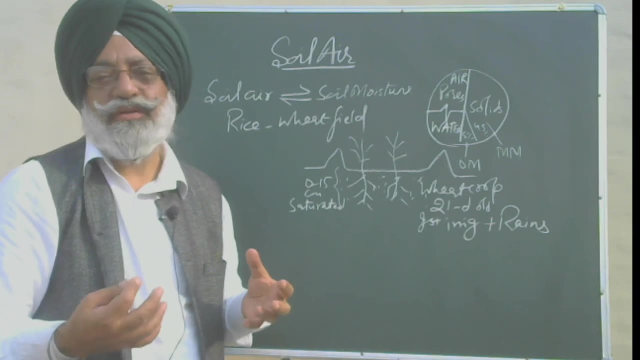 And if there is not any air, these plant roots won't be able to respire. If they are not able to respire, not take up oxygen, they won't have energy to take up water and nutrients. Though water is present in suction quantities, nutrients are present in suction quantities. Still, the plant roots cannot uptake because these do not have energy to take up nutrients and water from the soil, With the result we see typical nitrogen deficiency symptoms on the plant leaves. So this nitrogen deficiency symptoms, despite of presence of sufficient nitrogen in the soil. it is because of the stress, what we call as aeration stress, And if this aeration stress prolongs for a longer period of time, then even the plant roots may die and the yield decreases. So because of this aeration stress, there will be decrease in the crop yield. 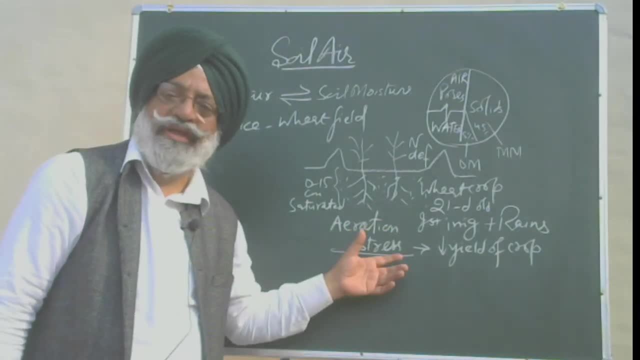 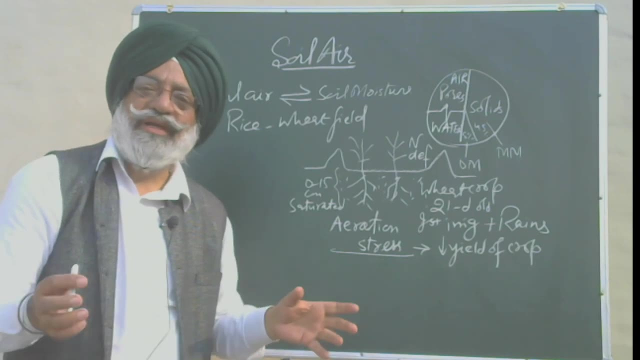 So this shows- now you might have a question over here that- why water loss conditions in 0 to 15 centimeters? Because it has been observed, particularly in coarse and medium textured soils, that because of continuous puddling of the soil, that means wet tillage. 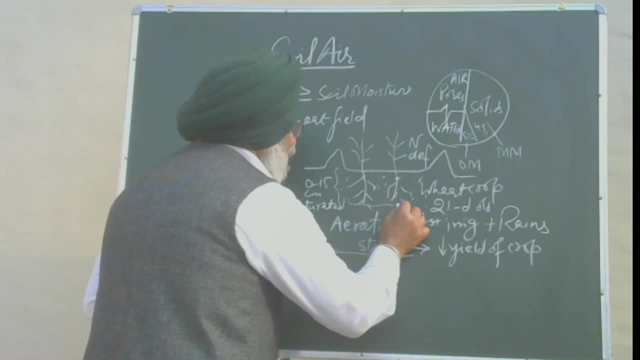 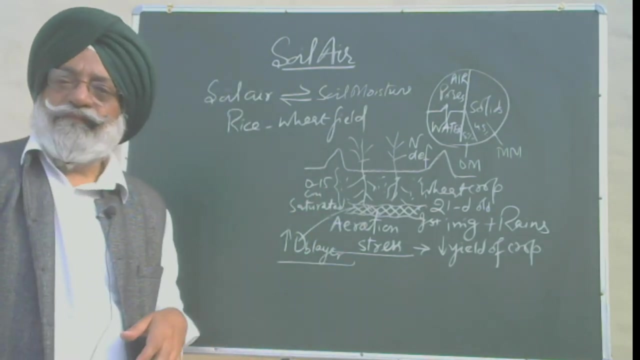 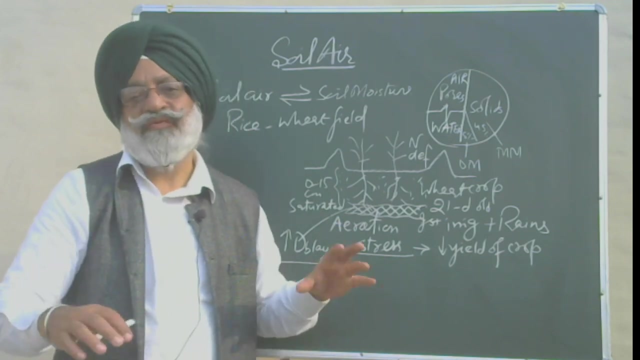 a sort of subsoil compaction is created over here. So this is high bulk days tillage. So this is high bulk days tillage which restricts the movement of water down into the soil, So deep drainage virtually ceases, and that's why this zone becomes saturated. There is deficiency of oxygen. what we call as aeration stress Plant shows nitrogen deficiency symptoms. So if you don't take the remedial measures, then even the crop yield roots may die. crop yield may decrease sufficiently. So this is why soil air becomes important. 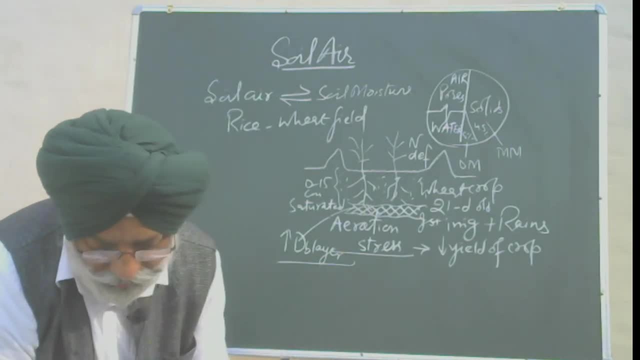 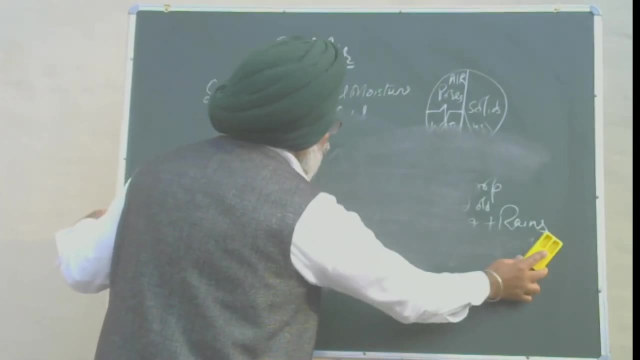 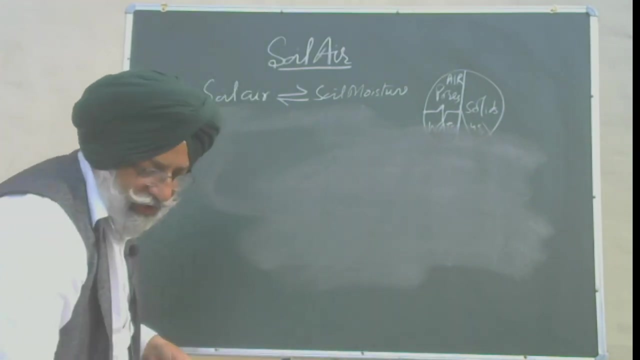 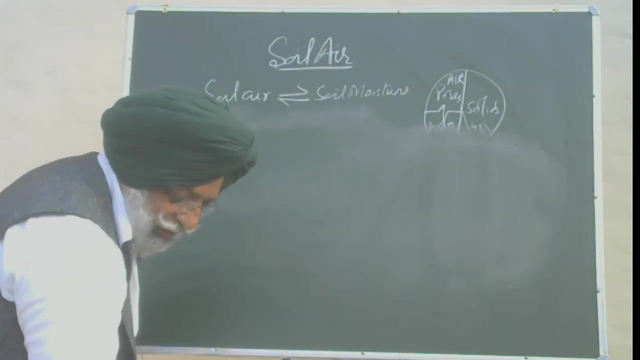 So soil air is, I should say, a very important component. So that's why we need to study this aeration. What is the mechanism, What is the composition of soil air, How we can, you know, manage soil air under such conditions? 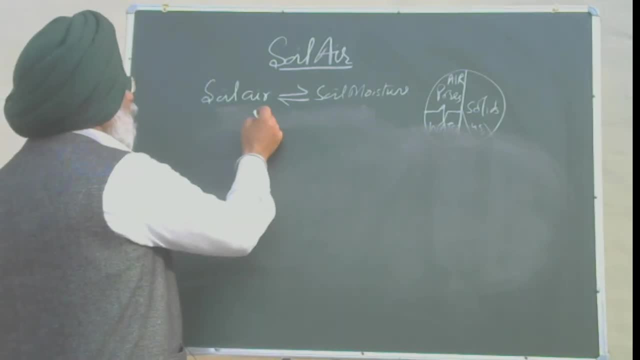 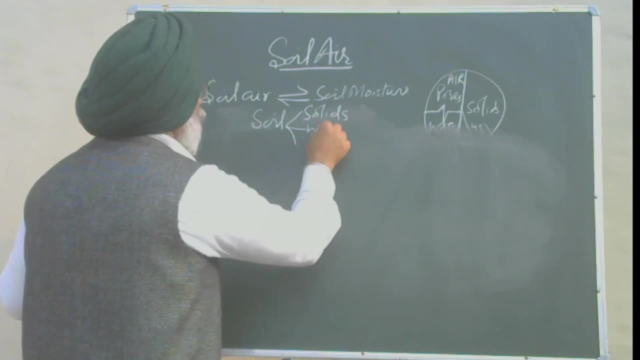 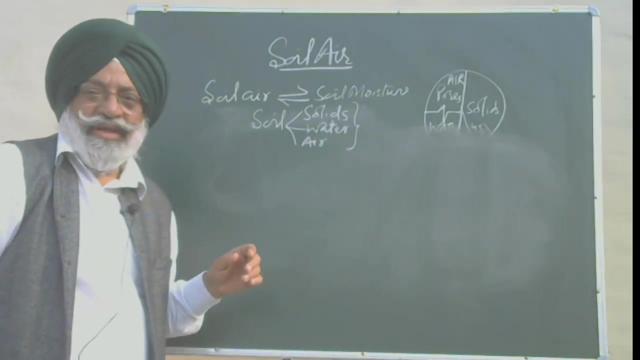 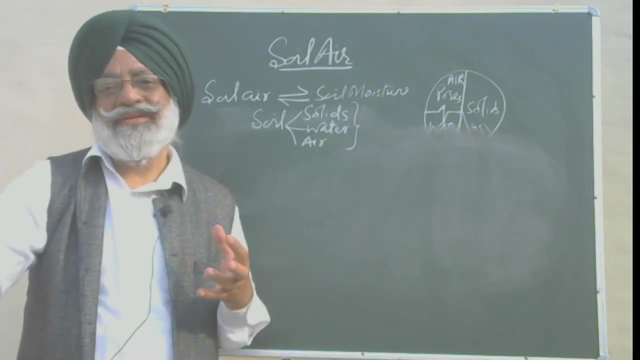 So, as I said that soil, you know it's made up of solids, Water and air or gases. So first of all, it's very important because, you know, if I see the soil, air, just like air in the atmosphere. it is compressible, you can compress it. So that means if we compress the air in the soil, the pore space will become empty. Number one: it's low density, of course, because just like air in the atmosphere, air in the soil is also low density soil and also low viscosity. 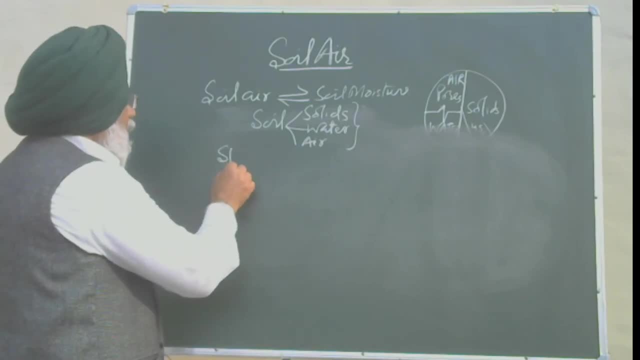 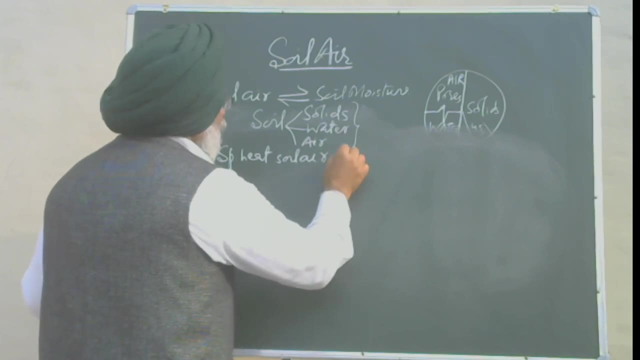 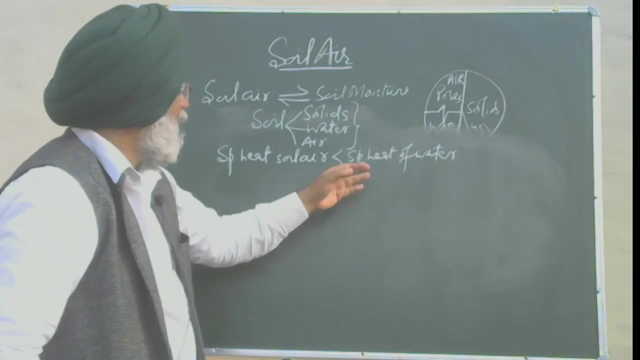 At the same time, the specific heat of soil air. soil air, you can call, or air that is less than that of specific heat of water. So we know this. So then it means if specific heat is less than that of specific heat of water. 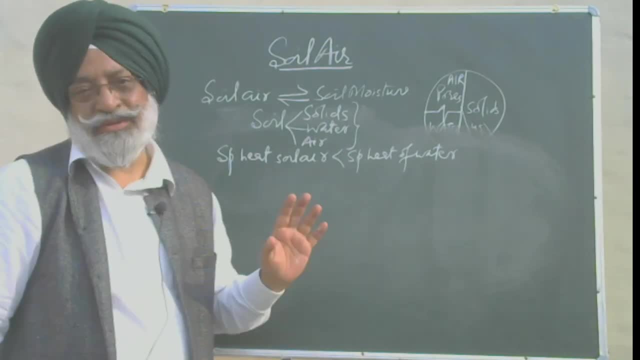 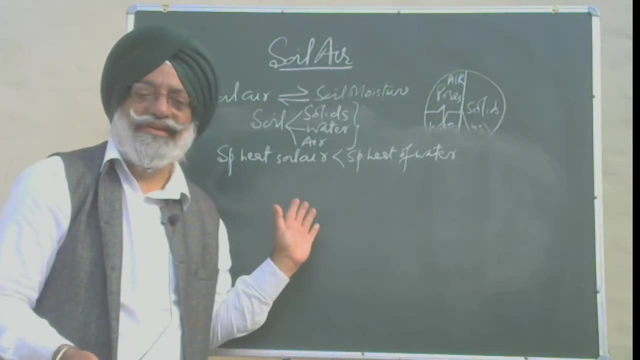 then of course, heat capacity of soil air will also be less than that, And you know specific heat: It is the amount of heat to raise the temperature of a particular substance, And here the substance is air through one degree centigrade. 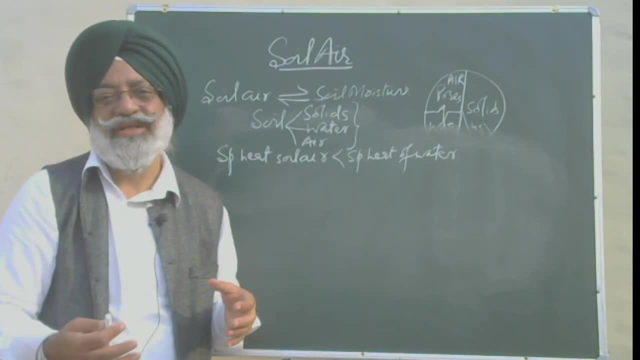 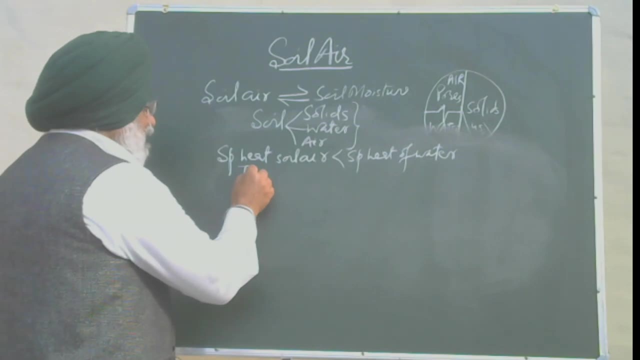 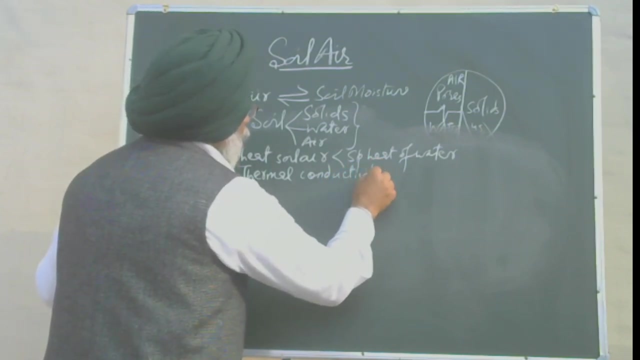 One gram substance. to raise its temperature to one degree centigrade, How much heat is required? That is the specific heat And also the thermal conductivity of soil air. Air is also low. Thermal conductivity of soil, air or air as such is also low. 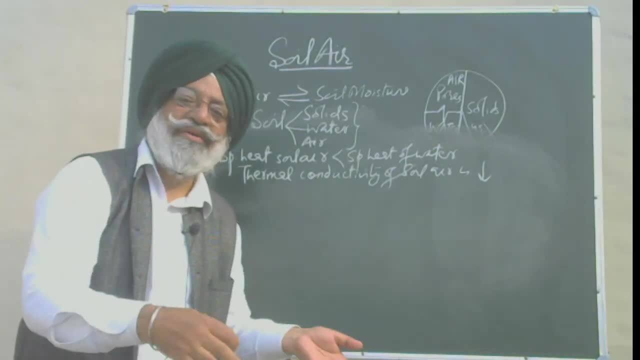 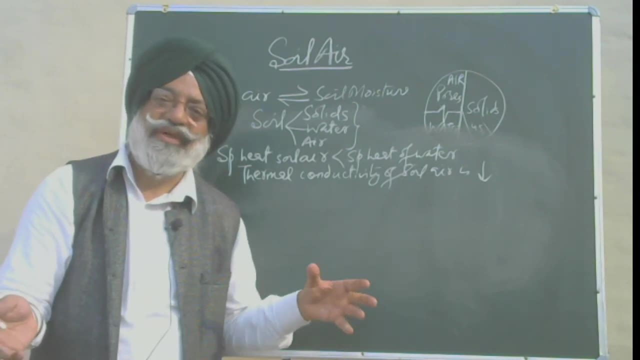 And you know, if thermal conductivity is low, the movement of heat transfer in the soil, that will also be dependent on, you know, the presence of air presence of moisture in the soil. higher the moisture content in the soil pore space. 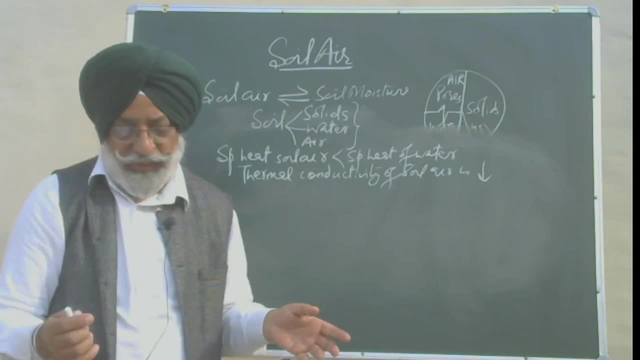 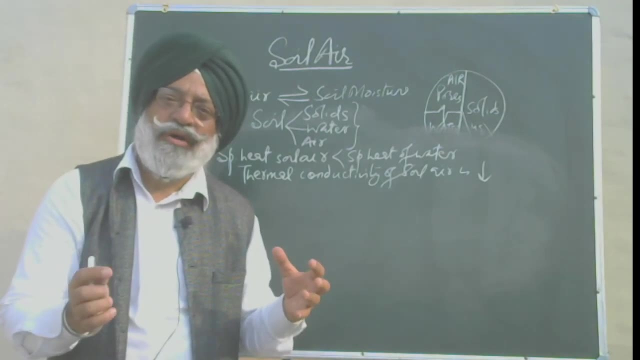 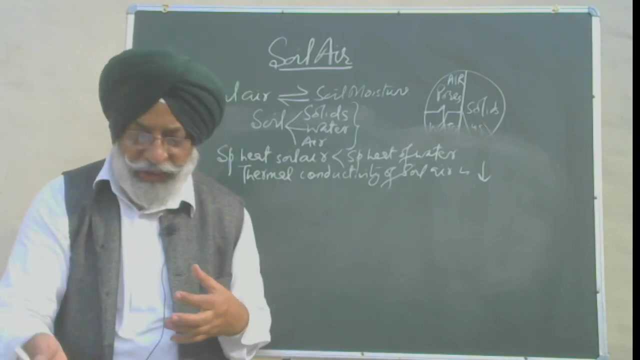 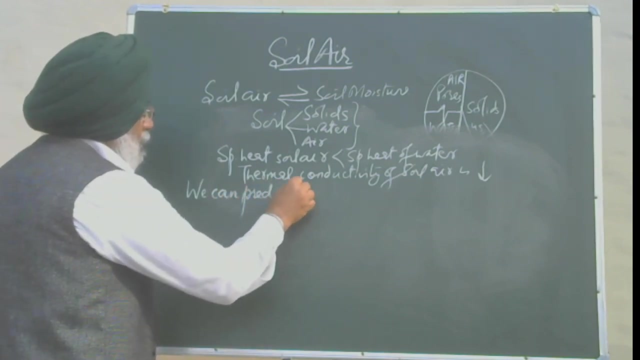 more will be. you know the transmission of heat through the soil. So, in nutshell, if you know the relative proportion of soil air or pore space occupied by soil air, then we can predict. So what we can predict? Number one: 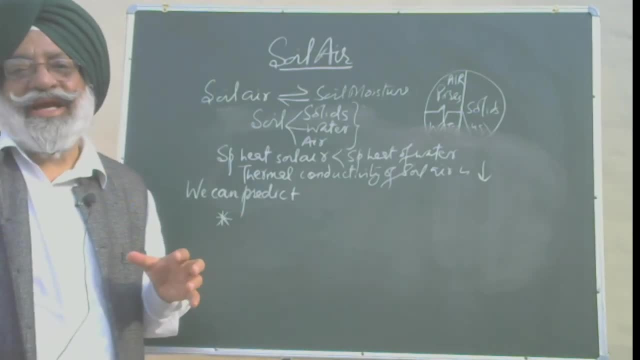 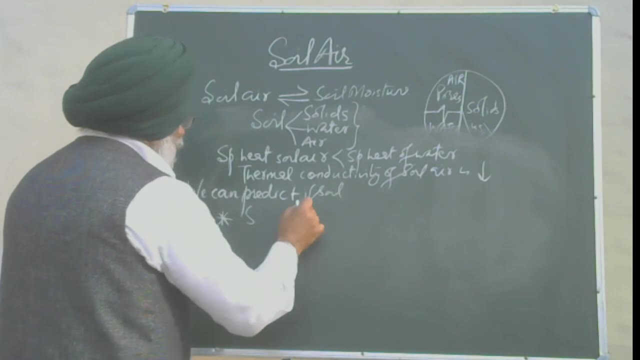 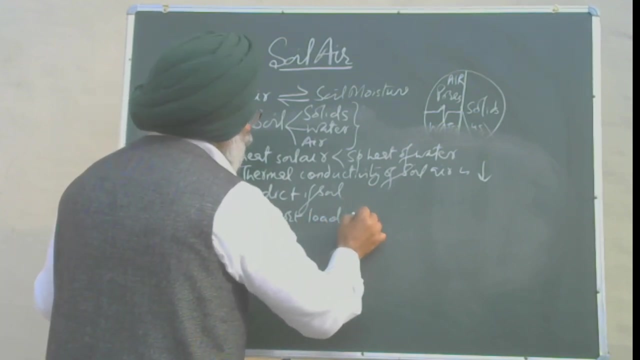 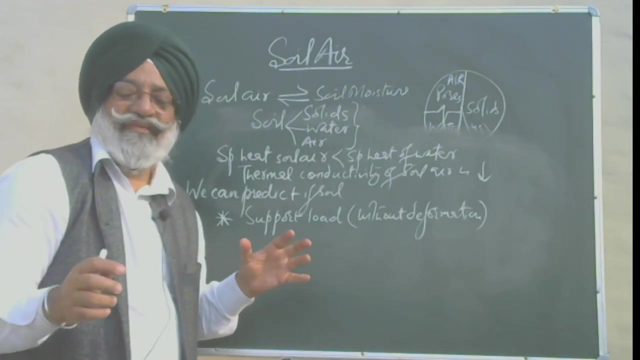 we can predict that, whether this soil can bear a load, Predict if soil can sport load. So when we say sport load, that means without deformation. So here again we have to see that whether this particular soil of which we want to know, 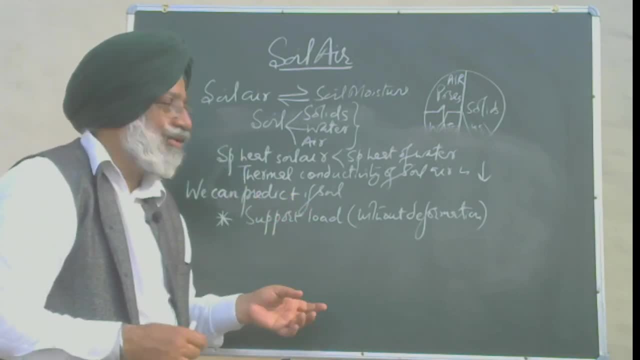 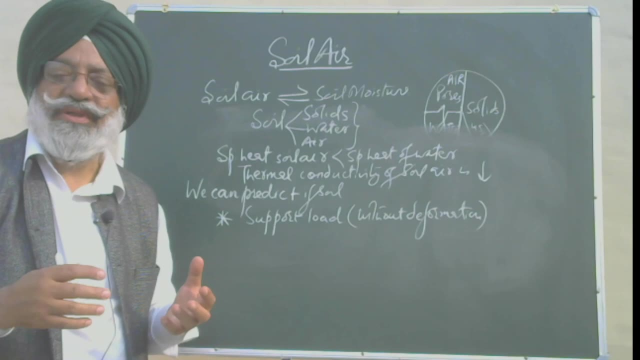 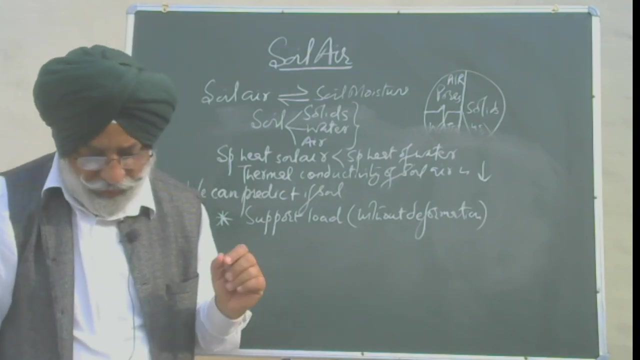 whether it will sport the load without deformation. it depends upon the pore space which is occupied by air. because air is compressible, So higher the pore space which is occupied by air lesser will be the capacity to sport the load. Number two: retain its shape When molding. Again, when you mold the soil, you are compressing it, and if there is more air space in the soil, then that means it won't be able to retain its shape when you put some external forces on it. 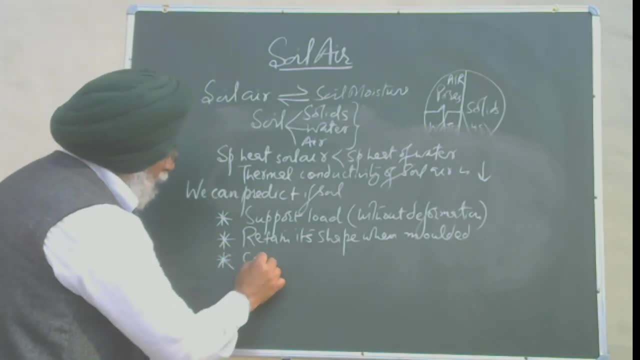 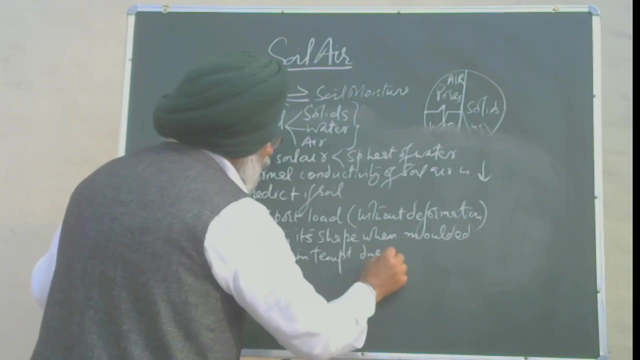 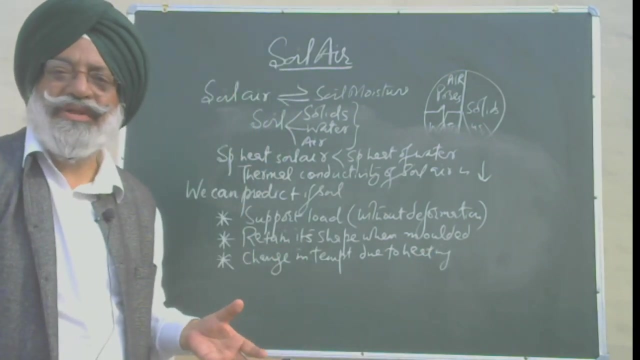 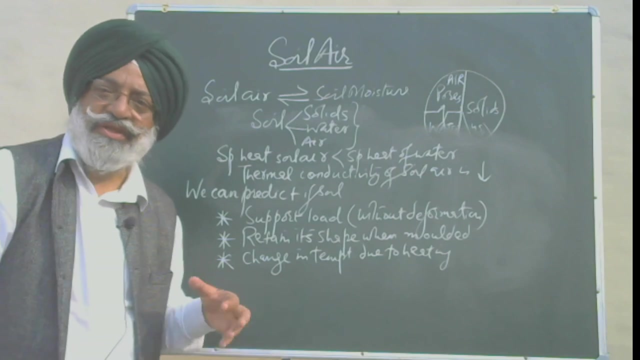 And third is change in temperature Due to heating. This is again very important. This heating could be because of the natural processes, the solar heat or maybe some artificial means. So if you heat the soil, how much change in temperature will be there? 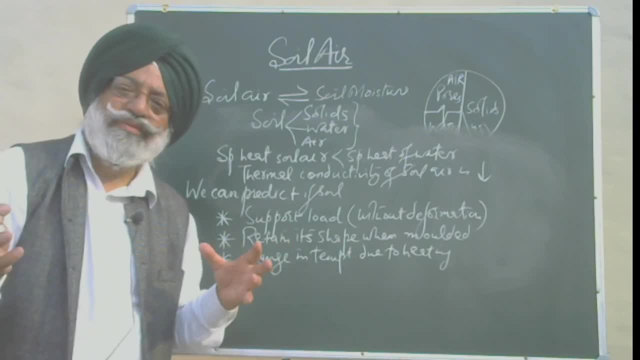 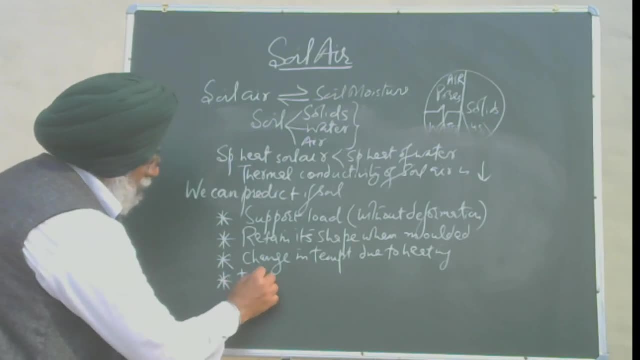 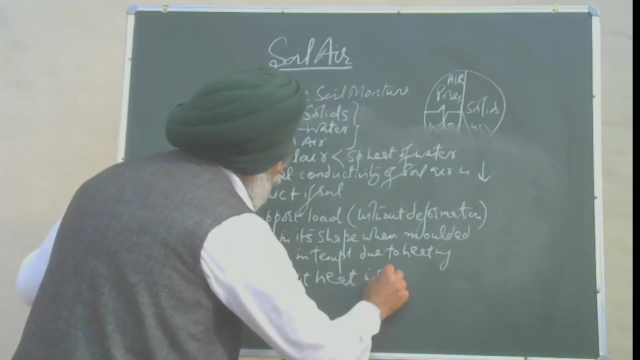 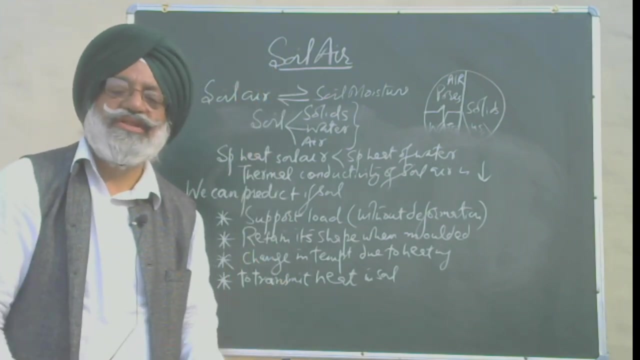 Again, it will depend upon the proportion of the pores occupied by soil, air And similarly to transmit heat. So that means if the heat radiations, thermal radiations, are coming from the solar system, they penetrate the soil. how deep this will go? 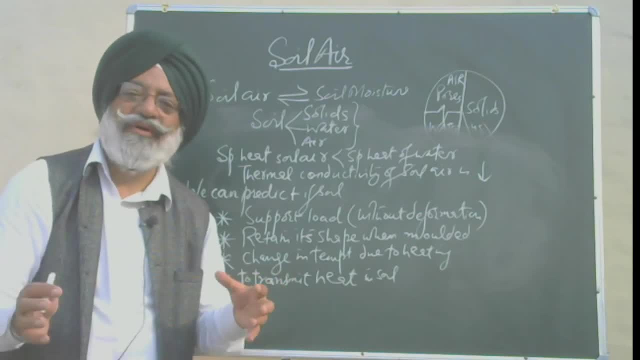 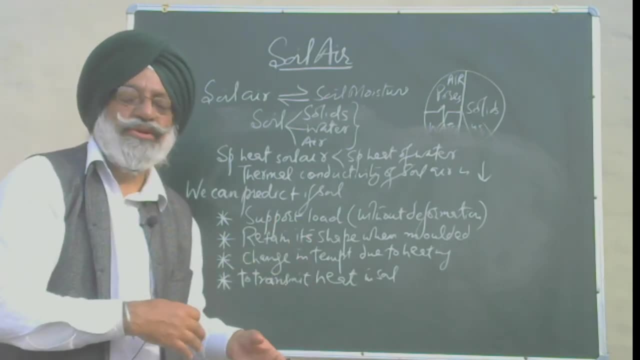 it will again depend upon the amount of, or the proportion of, pore space occupied by air. If you have higher amount of moisture than soil air, then this transmission of heat will be higher And, on the other hand, if you have lower amount of soil moisture, 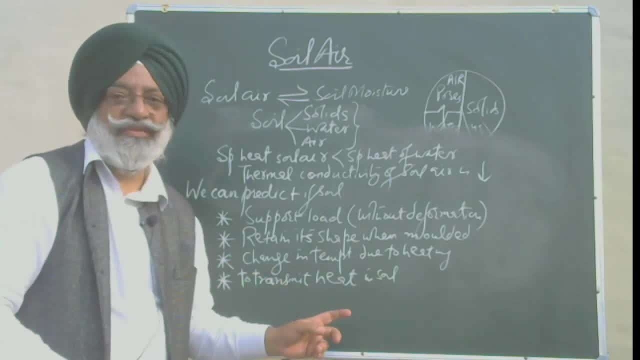 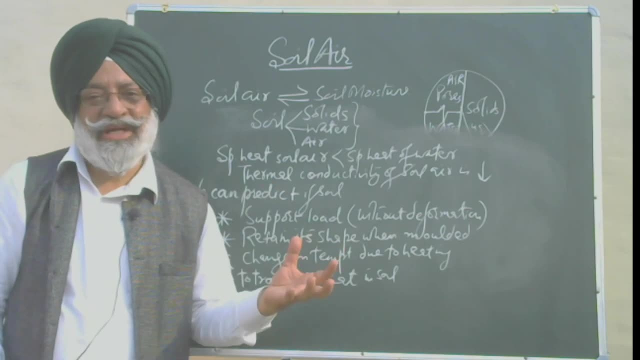 higher amount of soil air, then heat transmission will be low Because, as I said, the thermal conductivity of the soil is low. At the same time, specific heat of the soil air is low. Thermal conductivity of soil air is low, So it will determine. 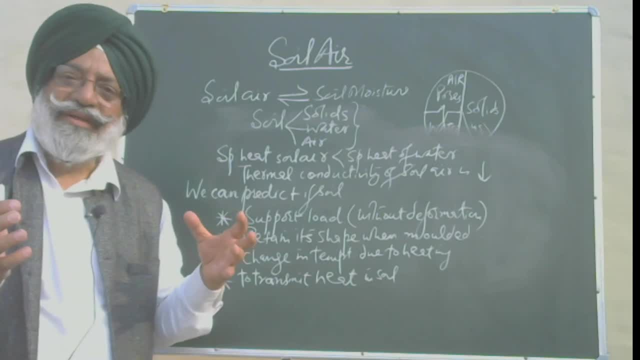 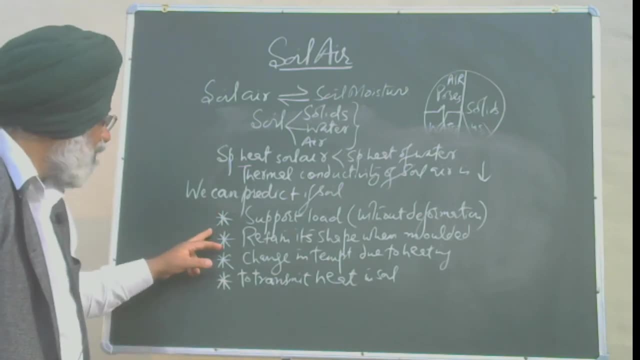 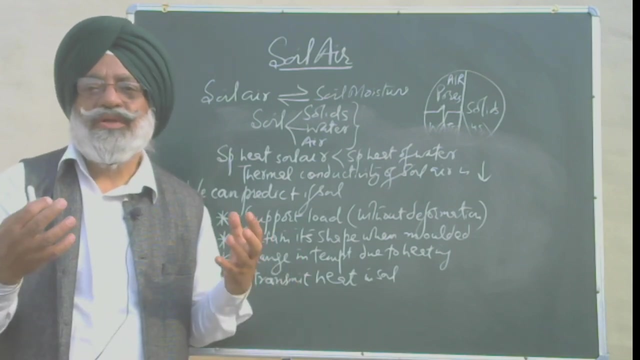 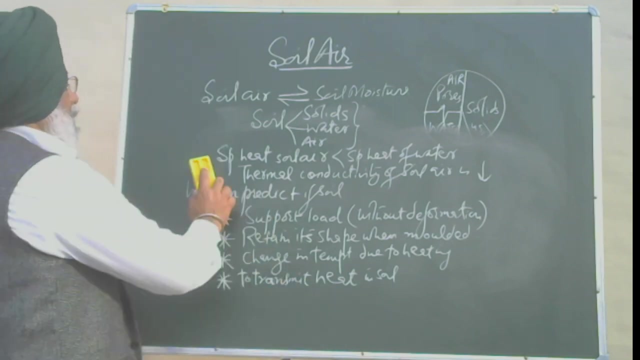 So you can predict, just knowing the proportion of soil air porosity or soil aeration porosity, you can predict these four things. So this is what you can infer from the air pore space of the soil. Then, coming to the composition, 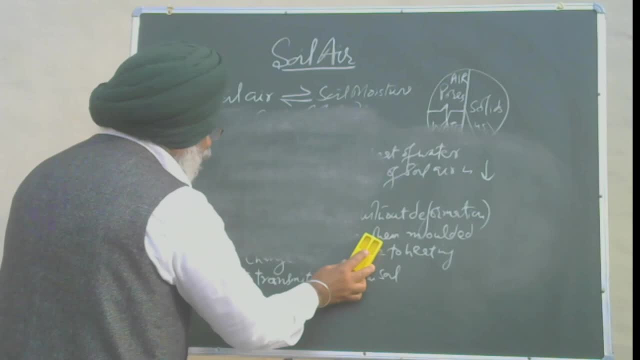 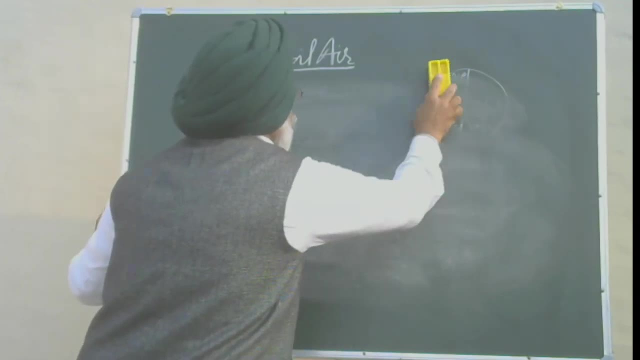 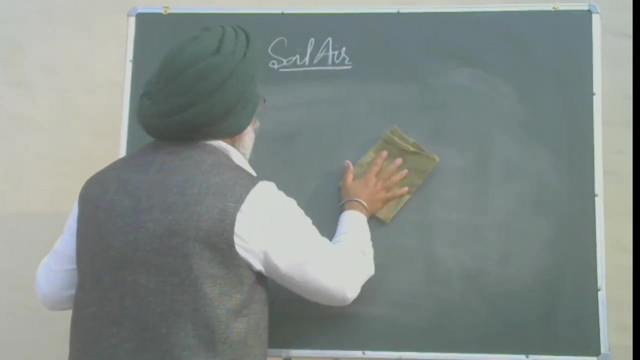 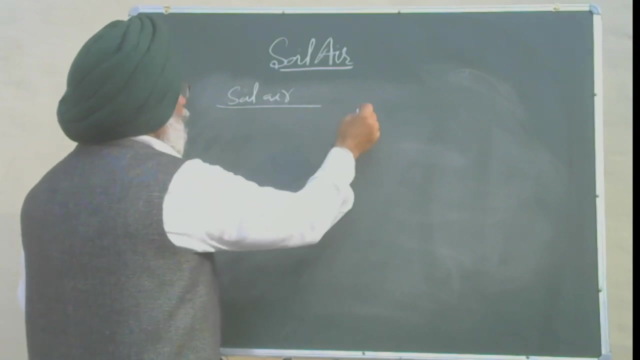 Is composition of soil air different from that of the atmosphere, or there is some difference? So we will just, you know, make a comparison over here. So on one hand we have soil air, On one hand, other hand, we have atmospheric air. So you know, the highest amount of the composition of air that is occupied by that contains nitrogen gas. So in atmosphere it is 79.2%- Is nitrogen. So 79.2% of the total- you know- volume of the air. that contains atmospheric, you can bet 79.0.. Whereas in soil air it is almost same: 79.2%. Then second important gas is oxygen, which is very important for the plant growth, particularly the plant roots in the soil. And you know this oxygen. I should say it is around 21%, Or you can say 20 point something, 7% in the atmosphere. So in soil it is quite variable. It could be as low as 5%. It could be as high as 20%. So it is very, very variable Depending upon so many factors. we will just now discuss what are those factors. Third, important gas is carbon dioxide. You know the carbon dioxide? it gets involved in the soil. First, because through the process of respiration by the plant roots, plant roots take up oxygen and give out carbon dioxide, So there is production of carbon dioxide. Similarly, microbial activities in the soil also produce carbon dioxide. They consume oxygen. So this is how. 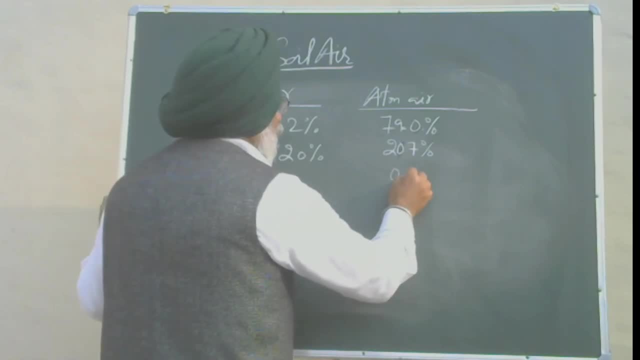 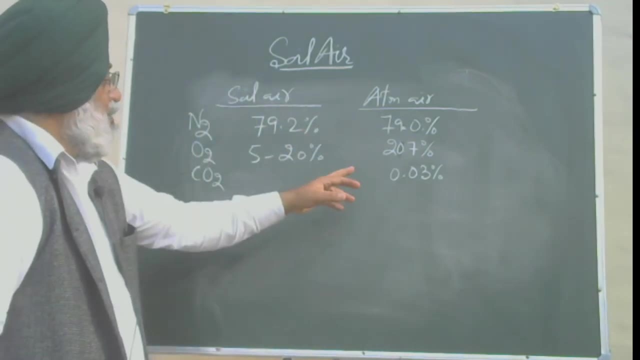 in general, the composition of you know here the amount of carbon dioxide present in the atmosphere is ideal. I am talking of ideal composition. So it is 0.03%. But in this case, in general, we say: 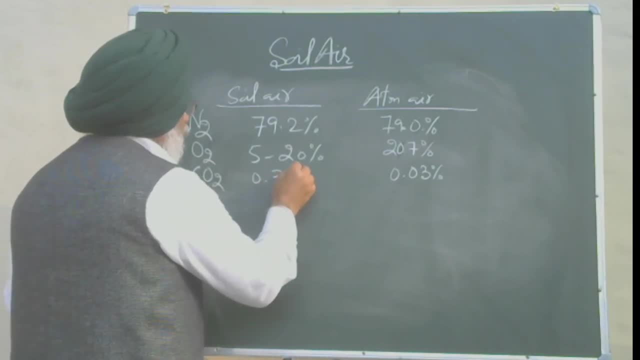 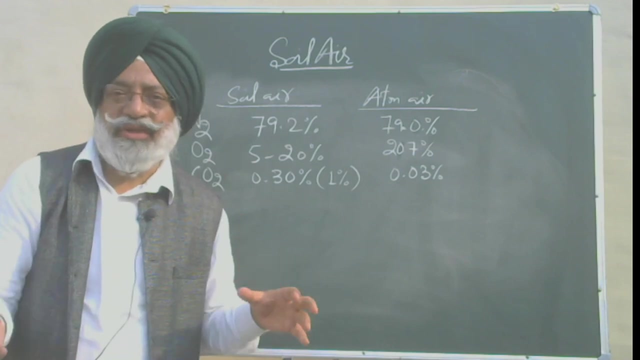 it is 10 times higher- 0.30%- But it could be as high as 1 percent, And 1 percent carbon dioxide means a lot, It is. it may affect the microbial activities in the soil. It may affect you know. 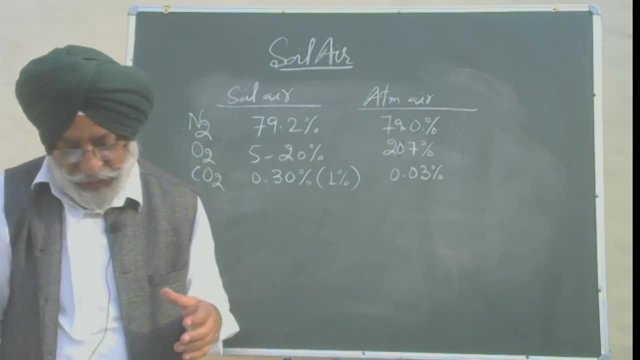 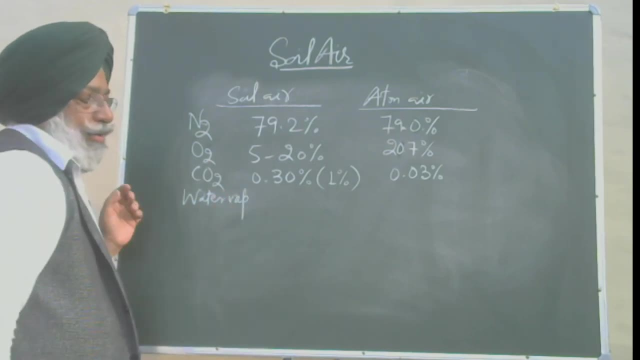 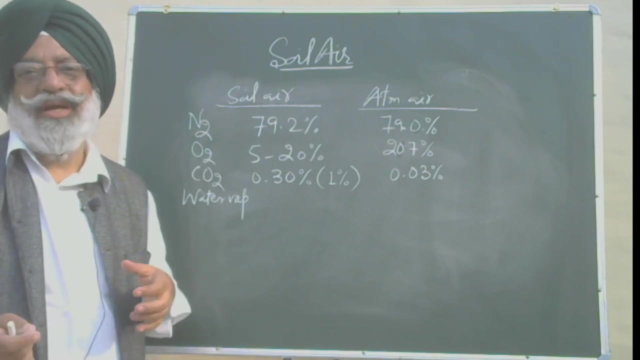 the plant roots, particularly in the soil. Then water vapors. that is also very important because water vapors in the atmosphere are it determines, you know, the amount of evaporation taking place from the soil, amount of amount of transpiration. 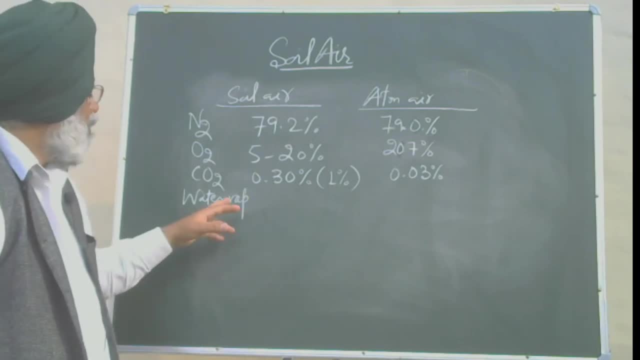 water transpiring from the plant leaves. So for that, the water vapor, it determines the relative humidity of the air. So these water vapors, these are, I should say are in soil, in because you know, 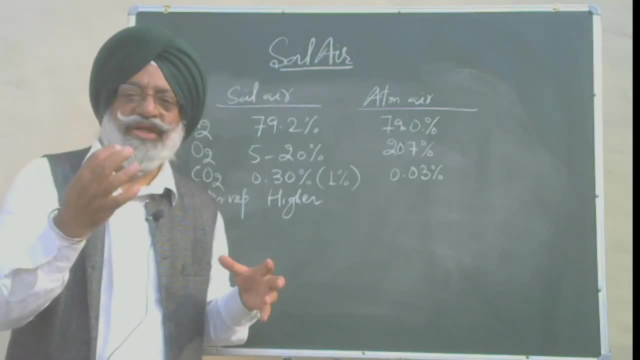 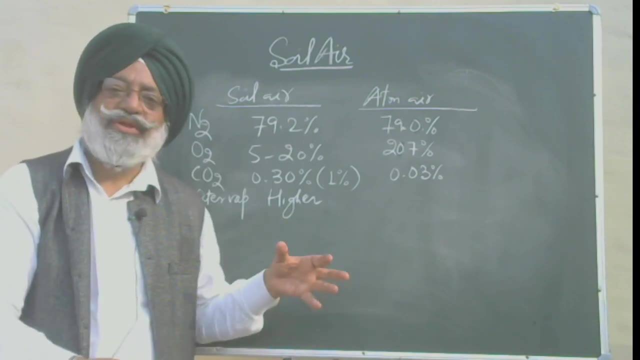 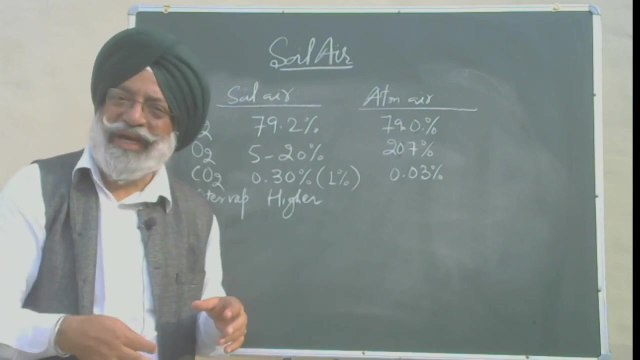 the air space. in the soil it contains, in general, macro pores, which are called water conducting pores, and micro pores, which are water retaining pores. So in general the water vapors they they are contained in the micro pores. 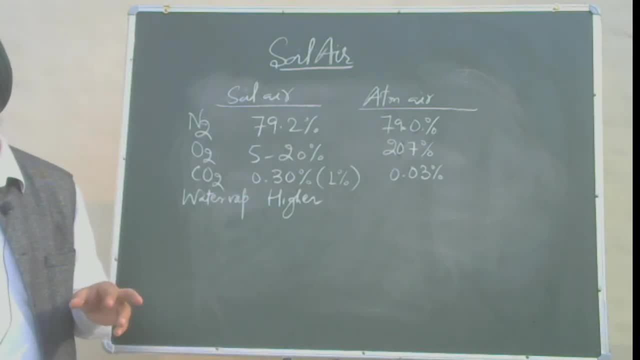 So higher the micro porosity, higher will be the moisture content in the soil, Whereas in the atmosphere it could be in places. Then here I should say the relative humidity of soil, air, it could be 100%. 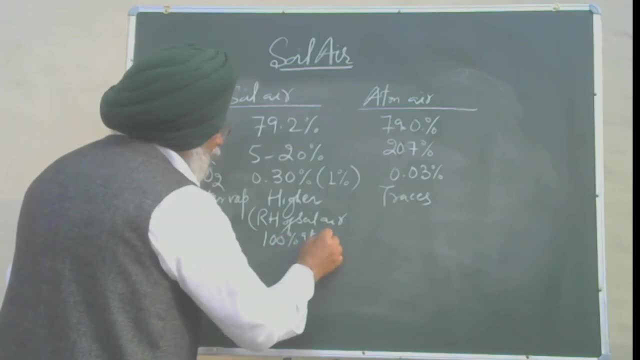 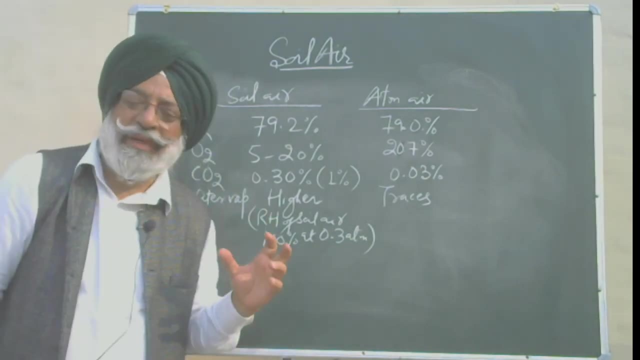 at 0.3 atmosphere of soil moisture content. And you know 0.3 bar or 0.3 atmosphere in fact is the water content available to the plants at field capacity moisture content. So if it is a field capacity, moisture content, the relative humidity of soil air could be 100%. So this is how the comparison is made. So this is how the comparison is made. So this is how the composition of soil air. it is different. from that of the atmospheric air. Now the question is: what are the factors which determine the composition of soil air? Factors affecting soil air composition are the following factors. The first is the composition of soil air, The second is the composition of soil air. The third is the composition of soil air. So here the first most important factor is flooding, When there are rains or when you irrigate the soil. so that means flooding is caused immediately after irrigation or immediately after. 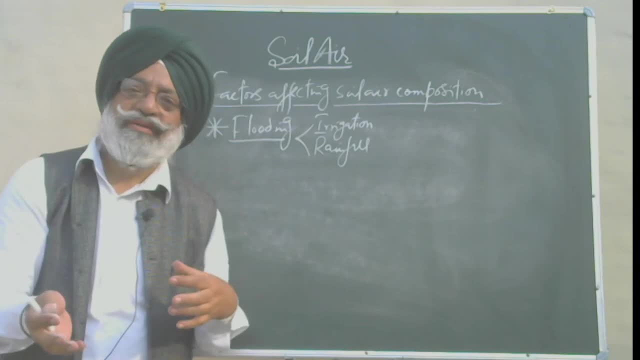 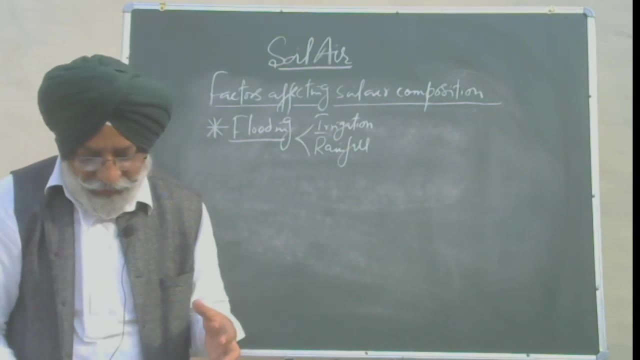 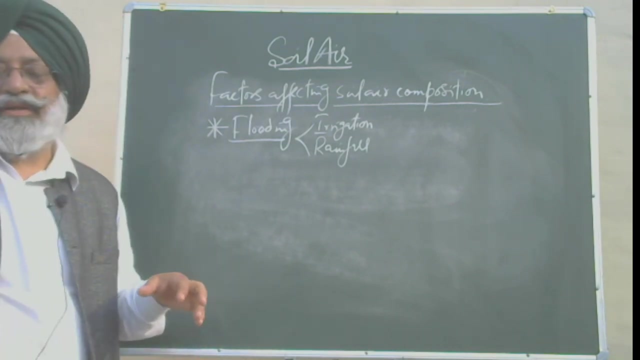 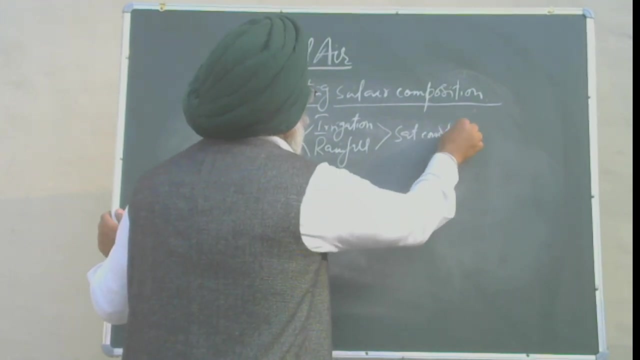 irrigation. So most of the air space in the soil it gets occupied by the moisture, by the water. So air in the pore space it gets replaced by the moisture or water present in the soil. And what happens then? due to that, 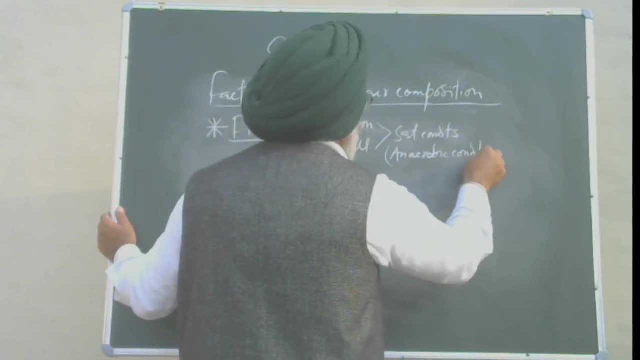 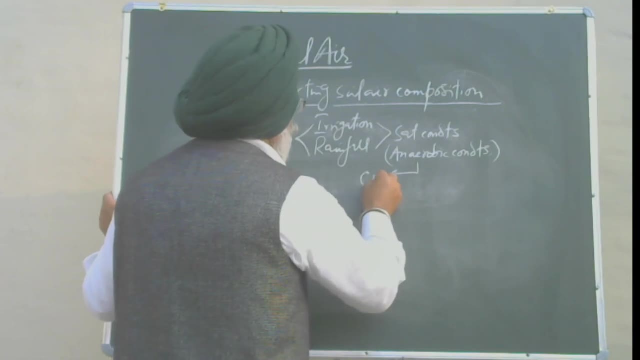 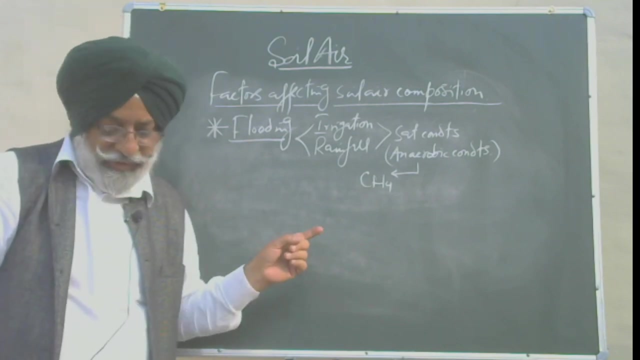 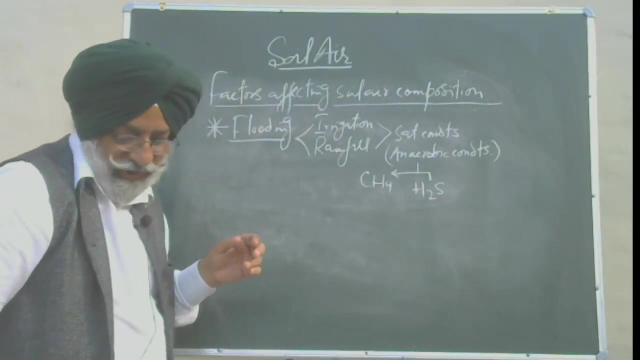 It leads to sort of anaerobic conditions in the soil And when anaerobic conditions are there, so that means you have production of methane gas, because when carbon decomposes in the absence of oxygen, it produces methane, You may have high content. 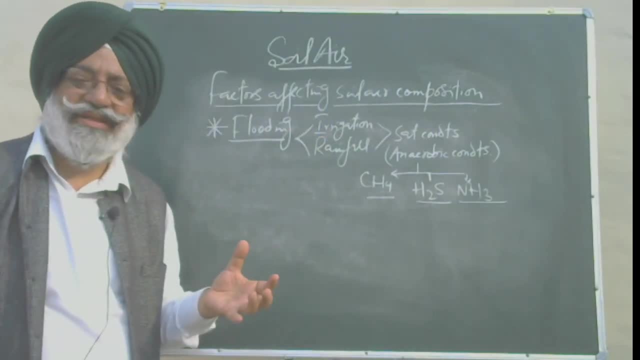 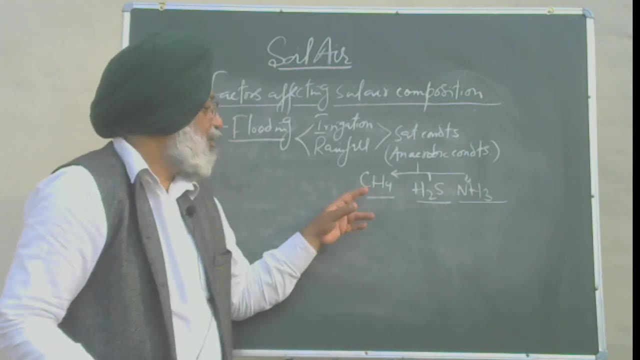 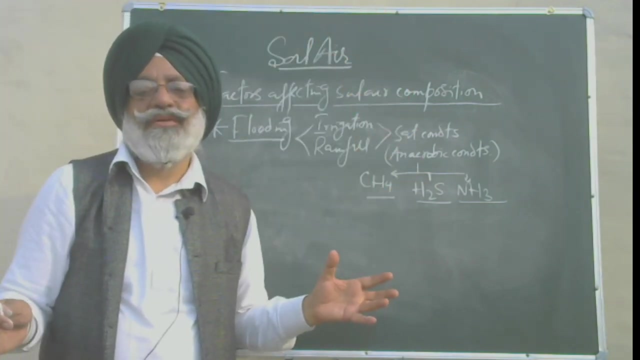 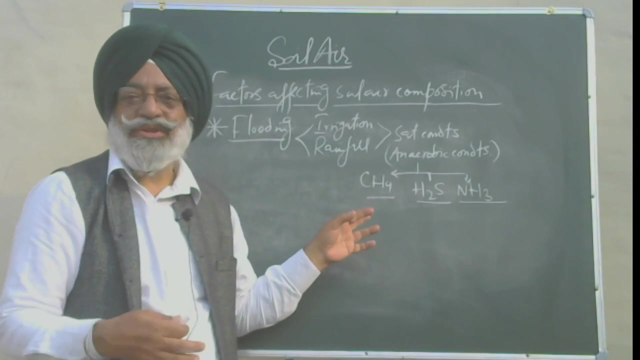 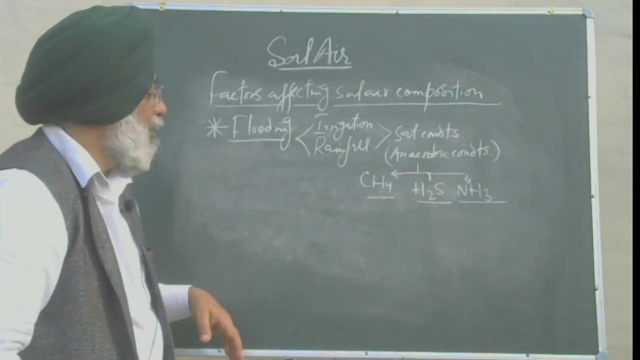 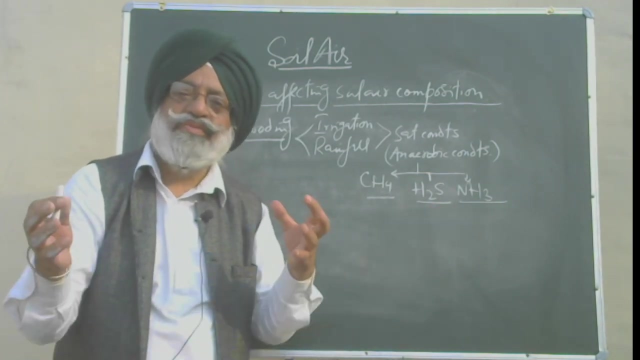 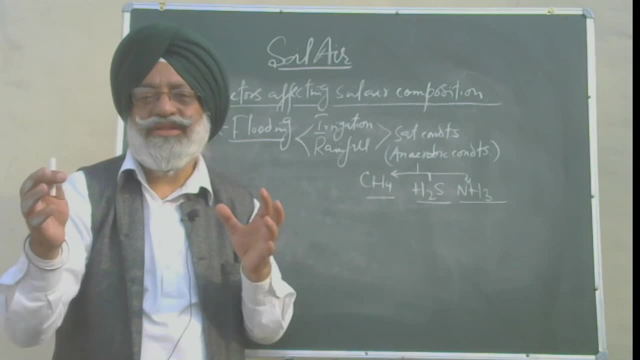 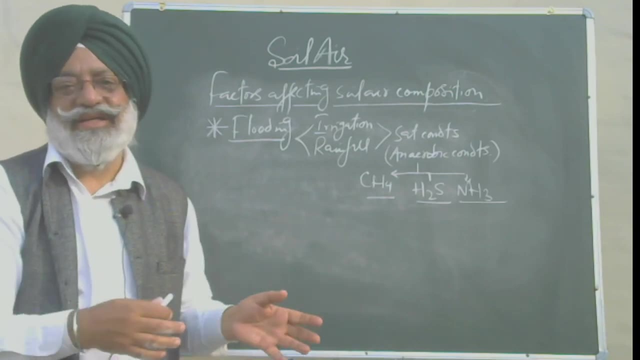 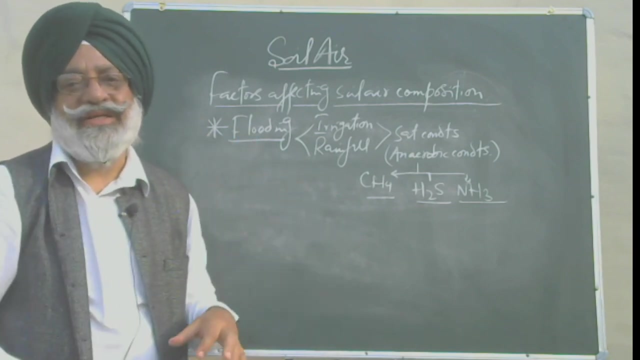 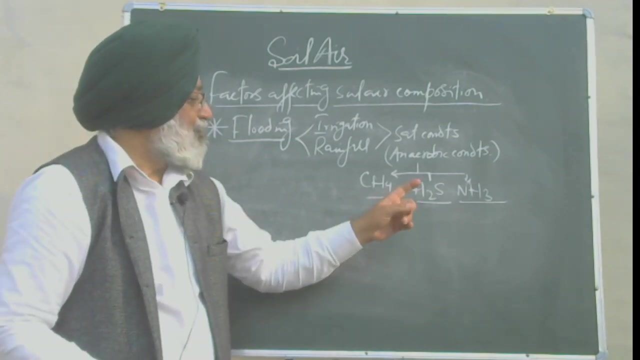 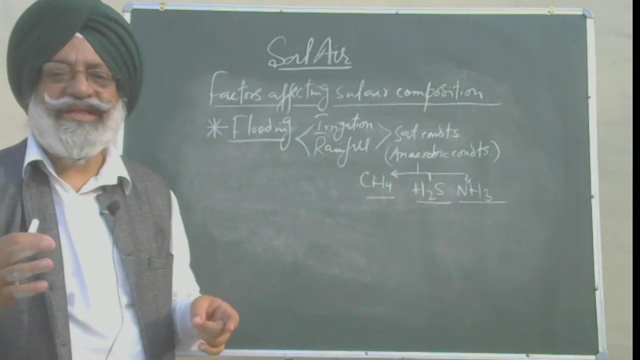 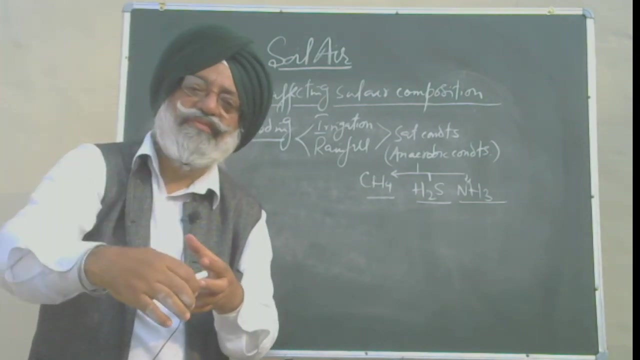 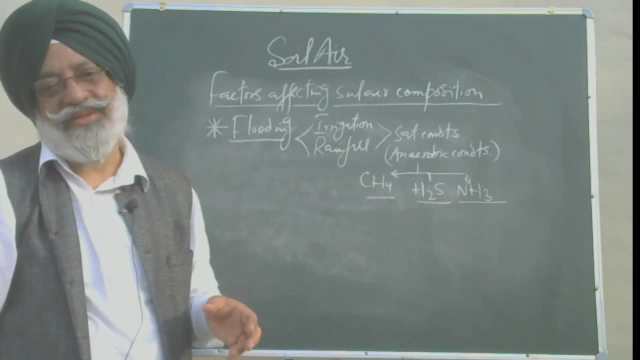 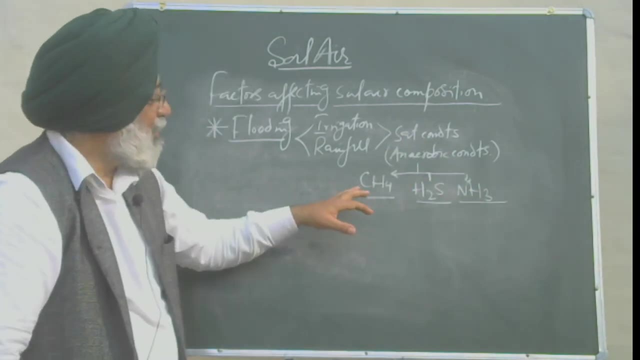 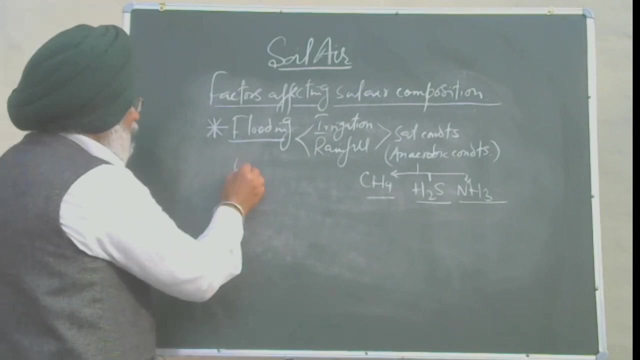 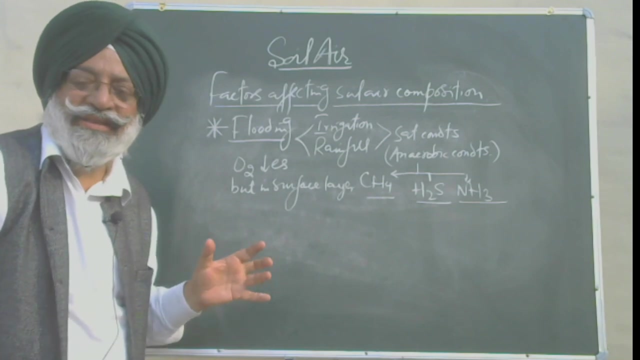 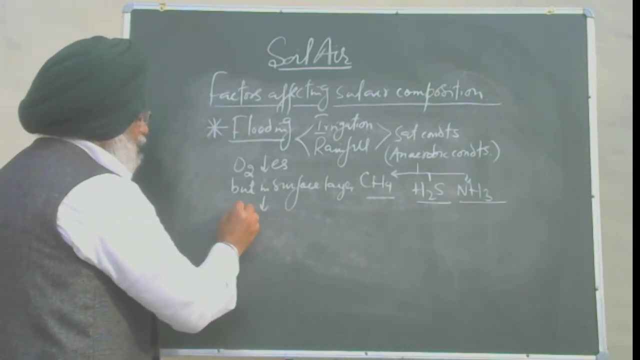 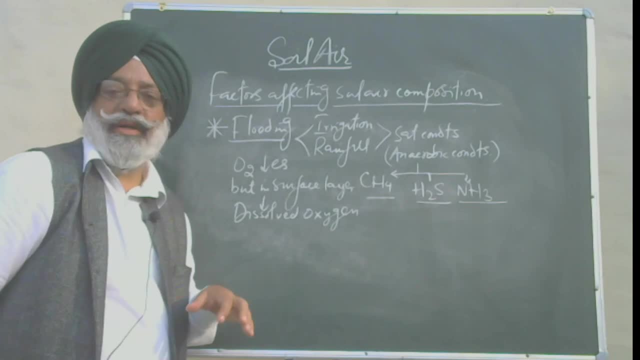 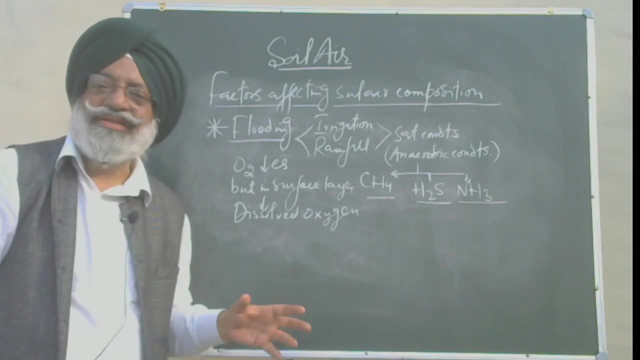 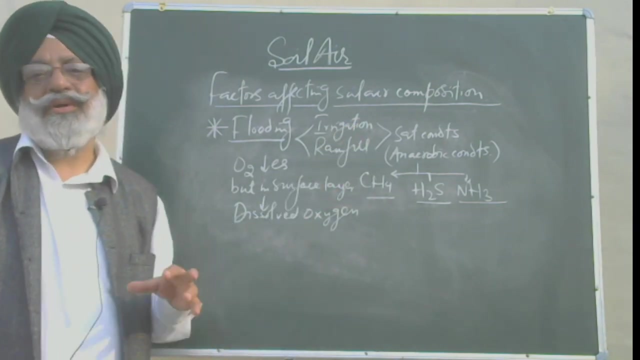 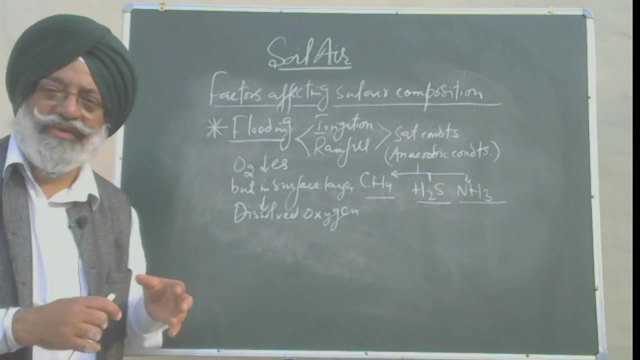 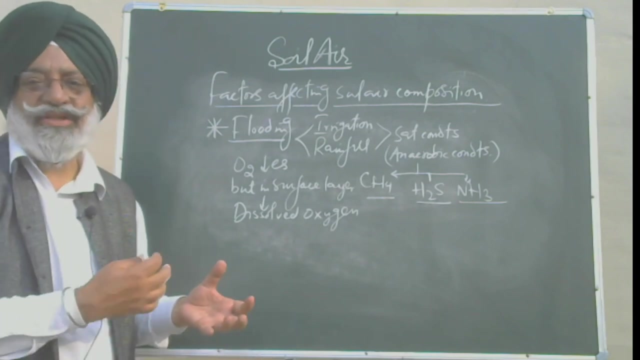 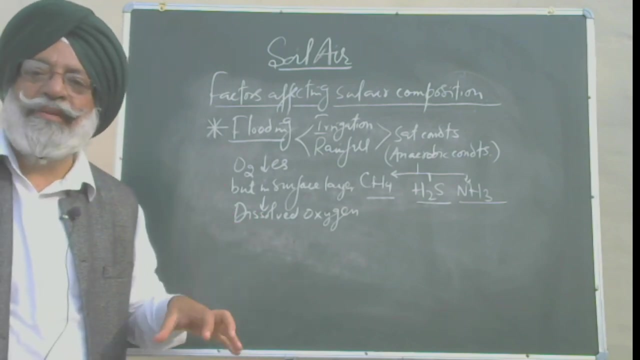 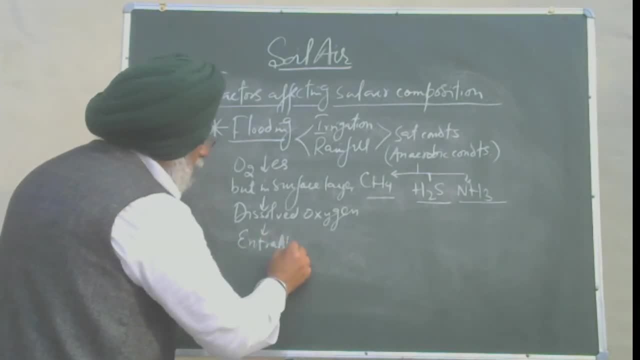 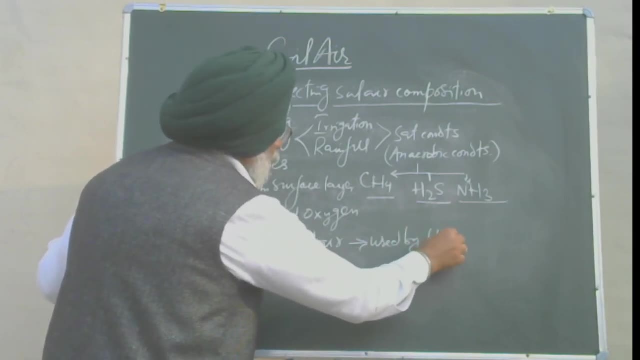 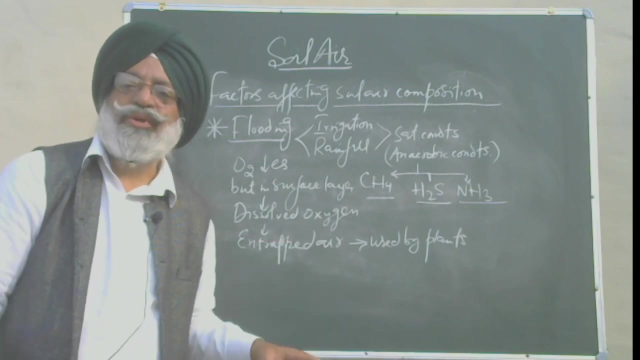 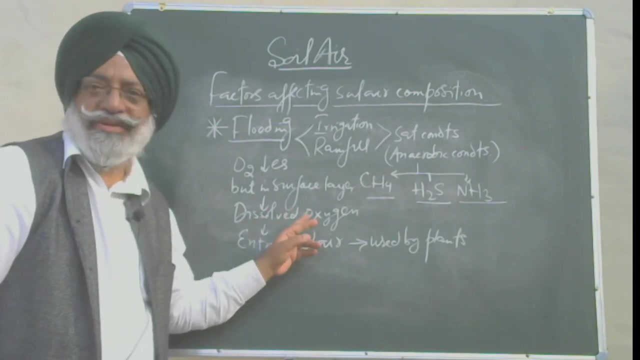 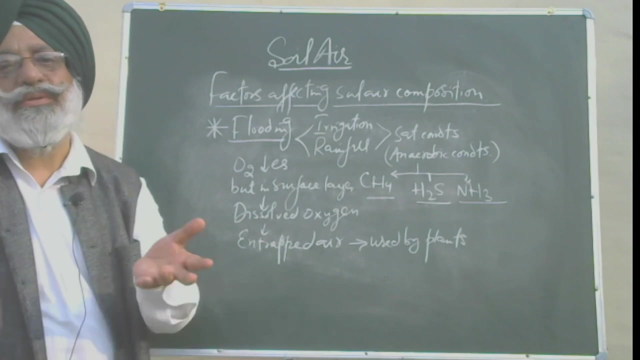 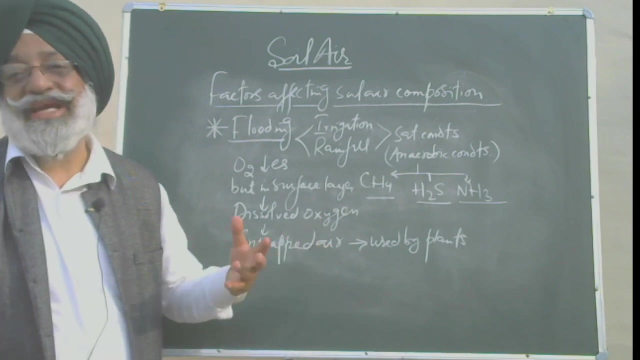 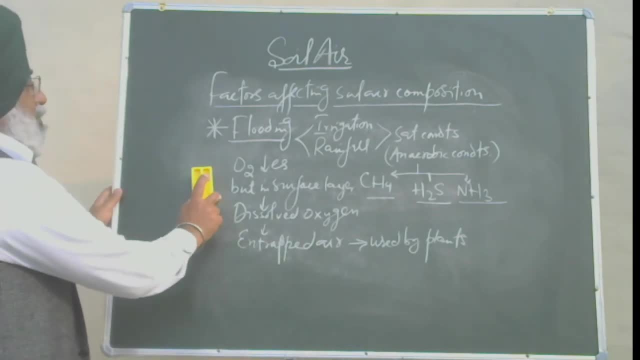 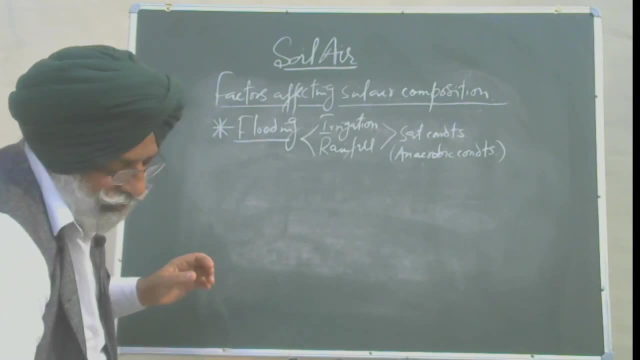 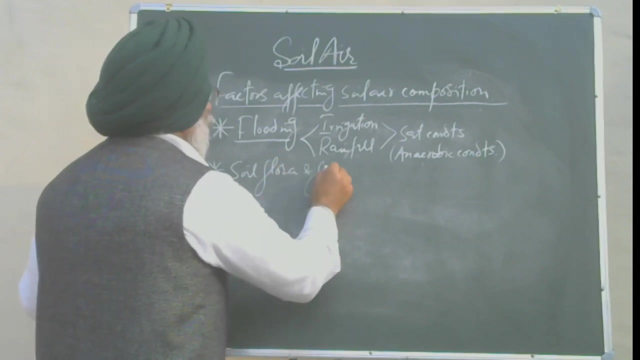 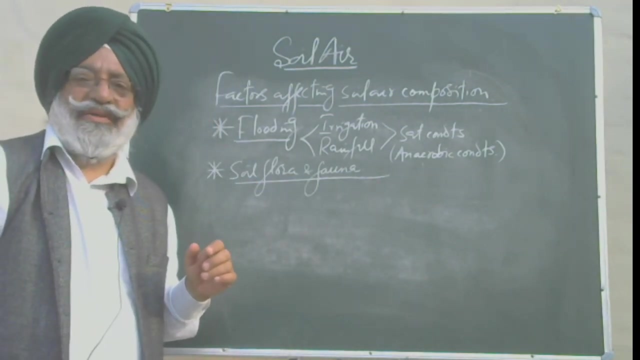 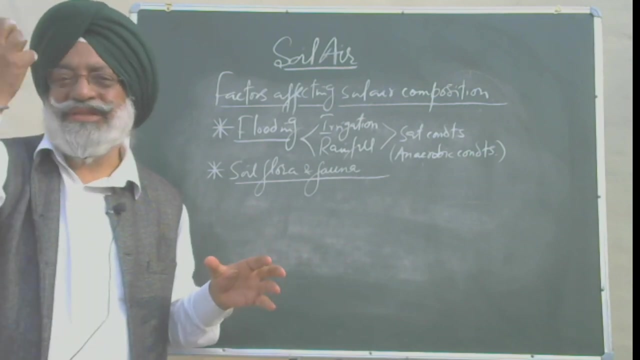 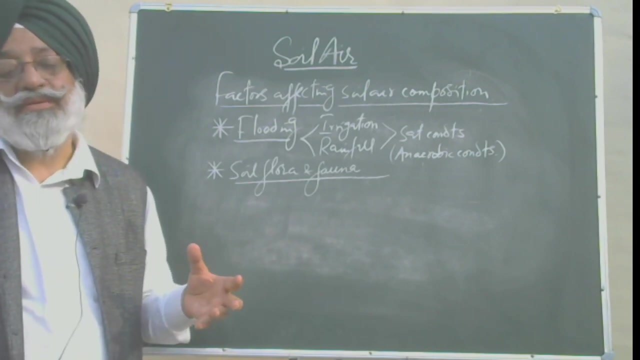 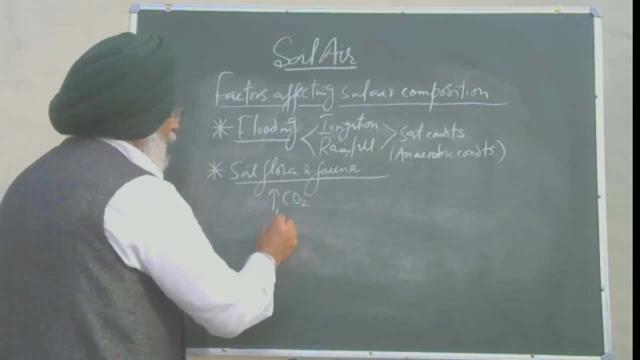 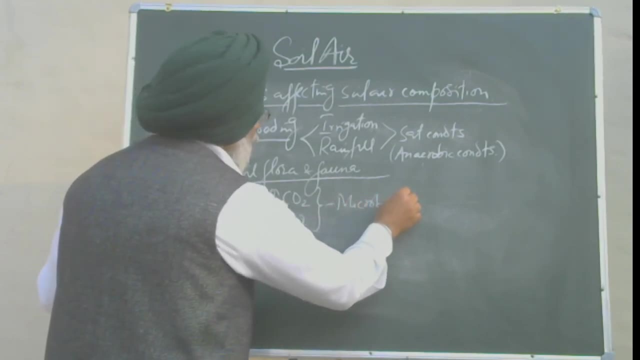 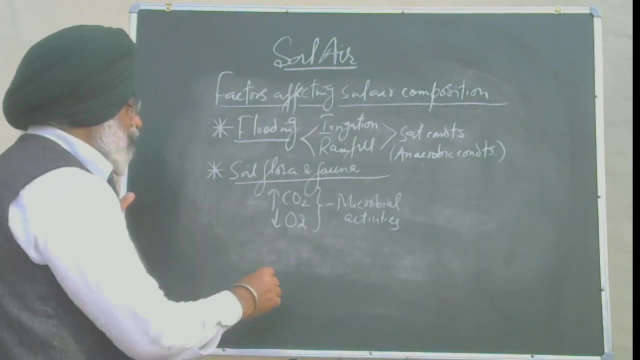 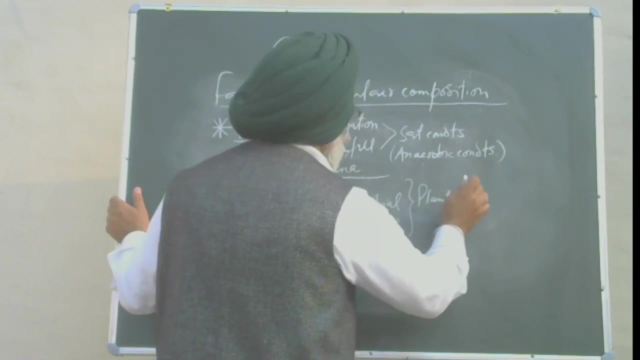 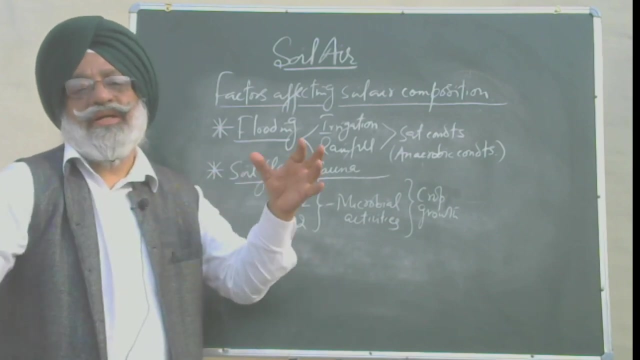 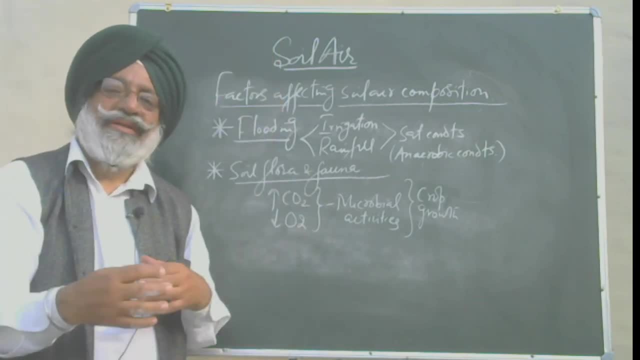 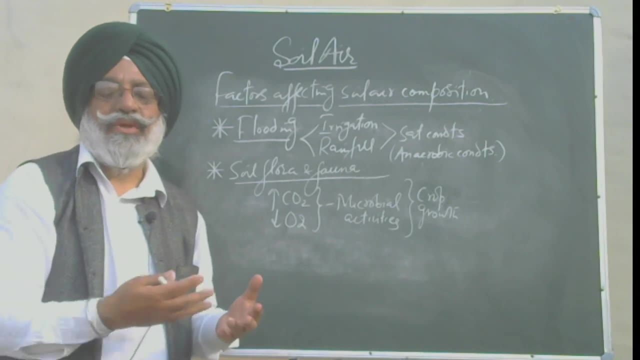 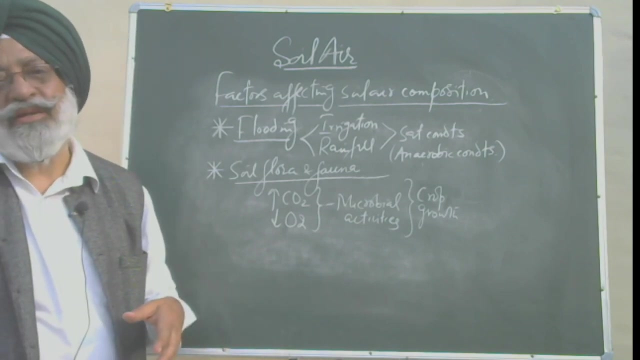 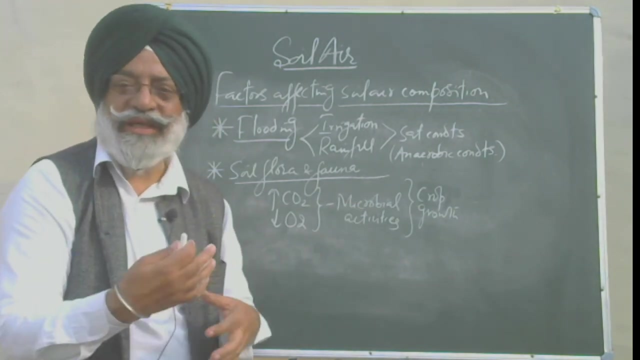 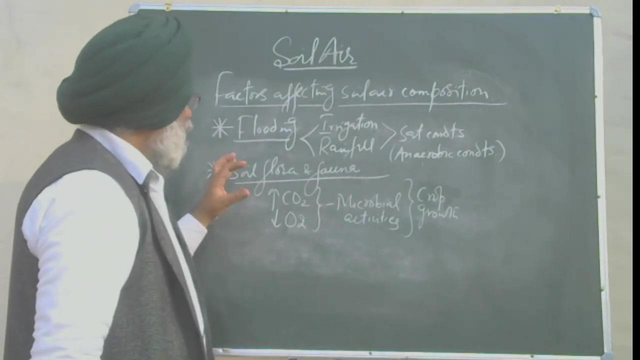 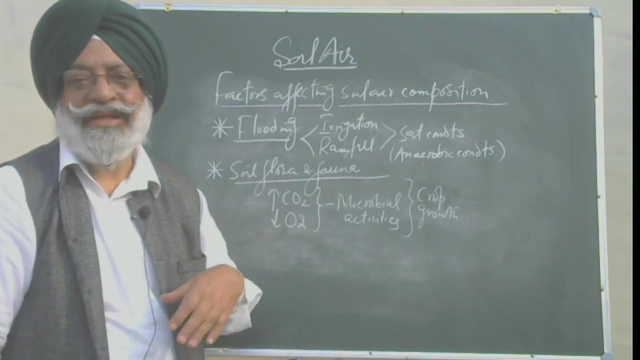 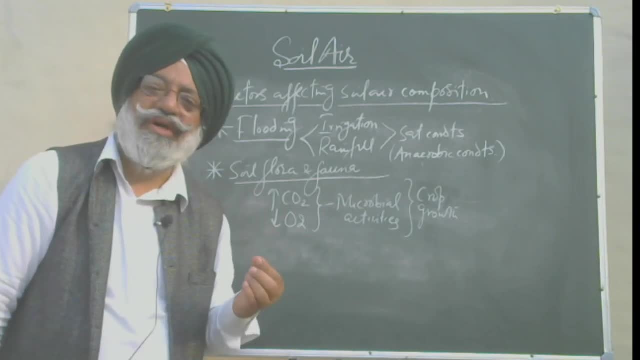 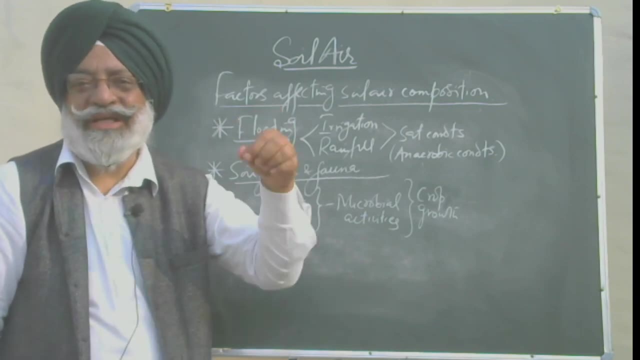 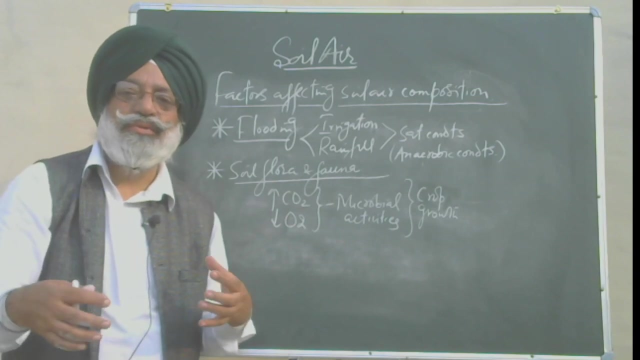 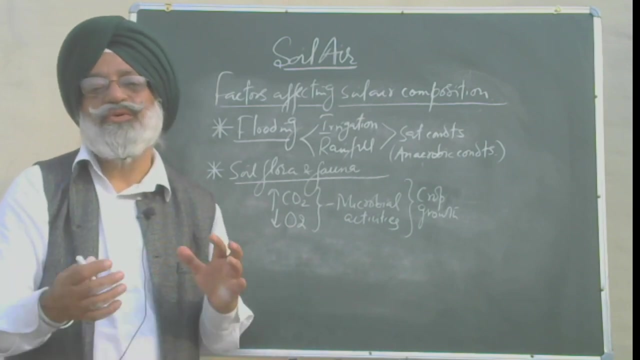 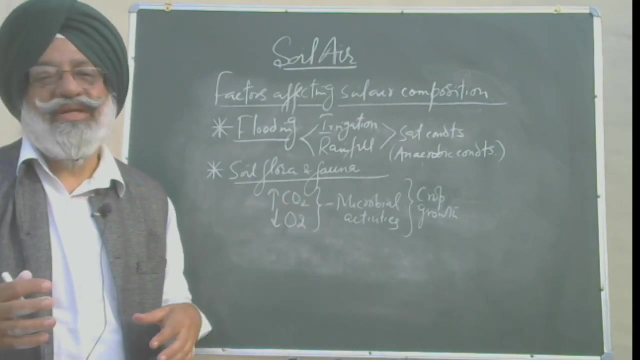 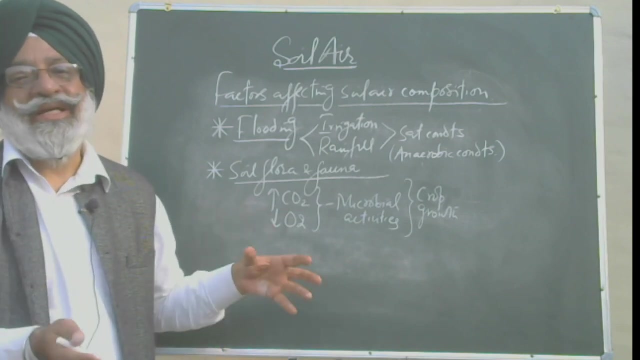 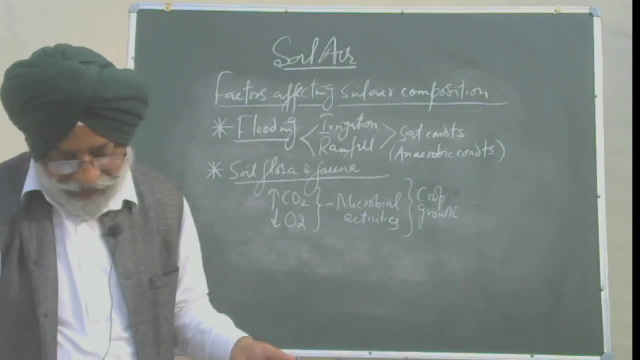 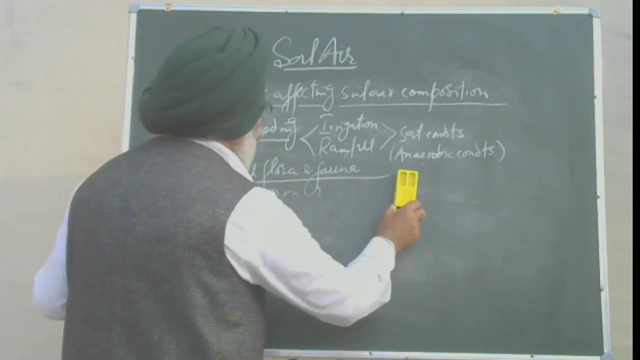 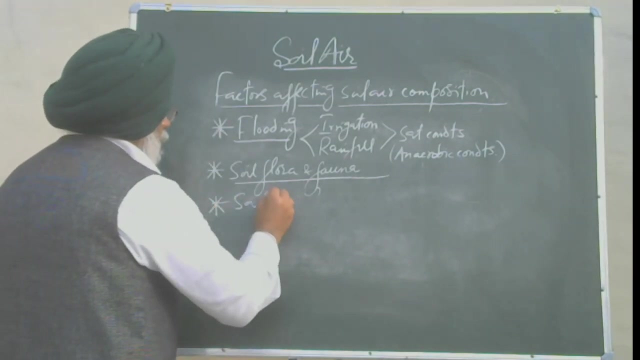 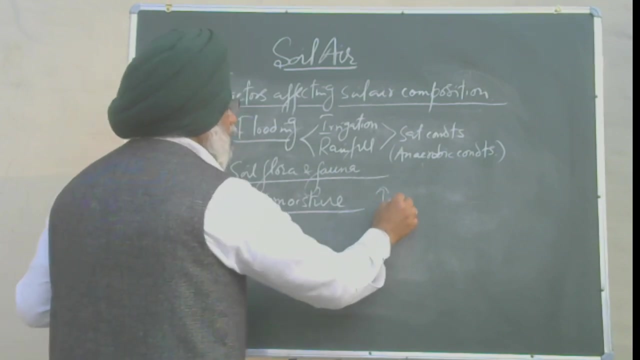 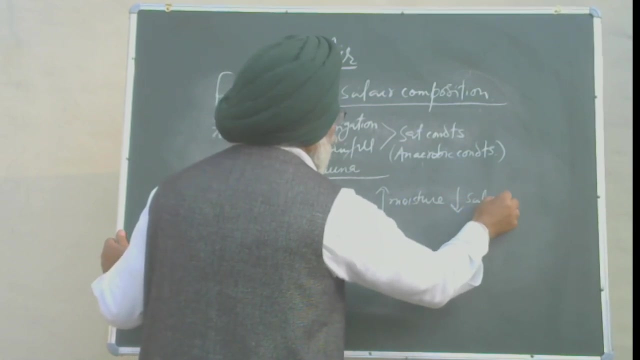 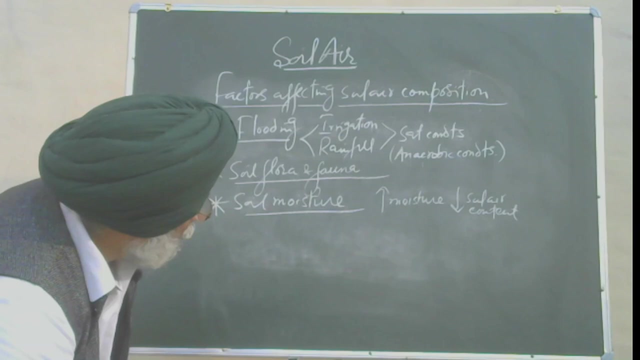 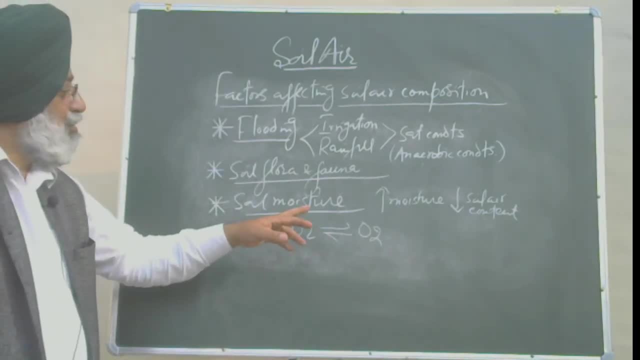 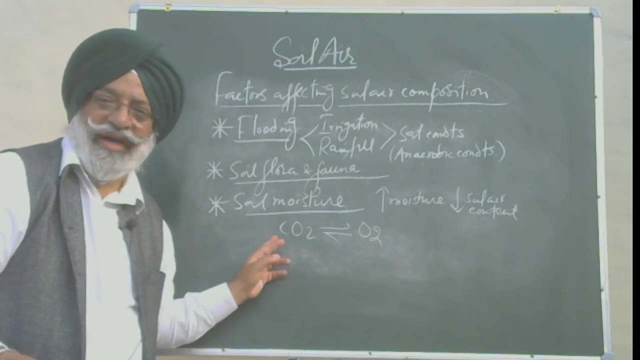 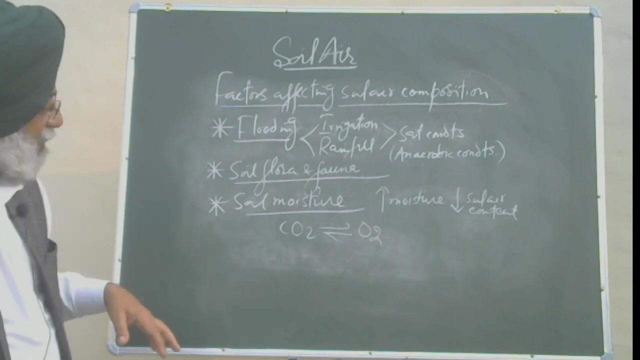 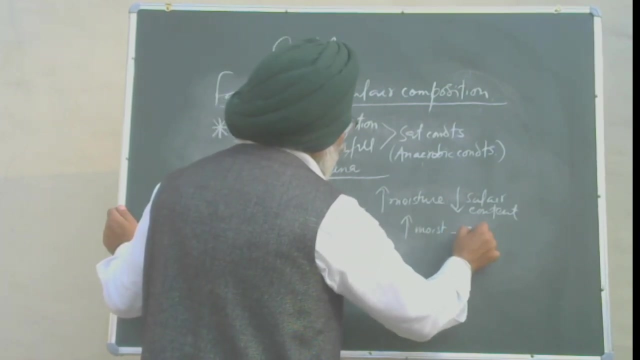 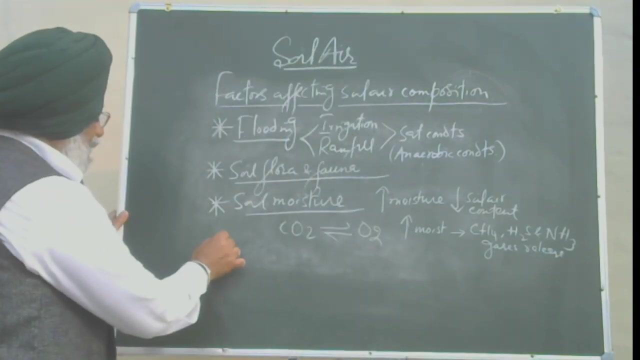 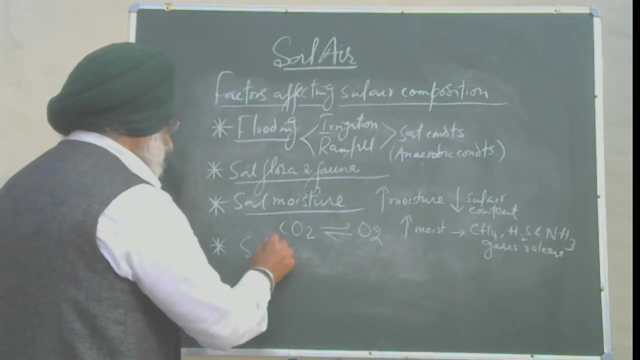 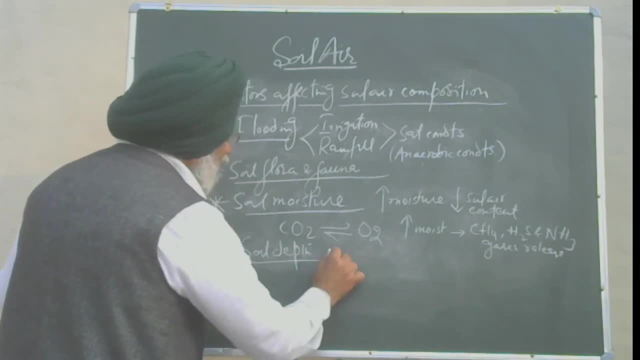 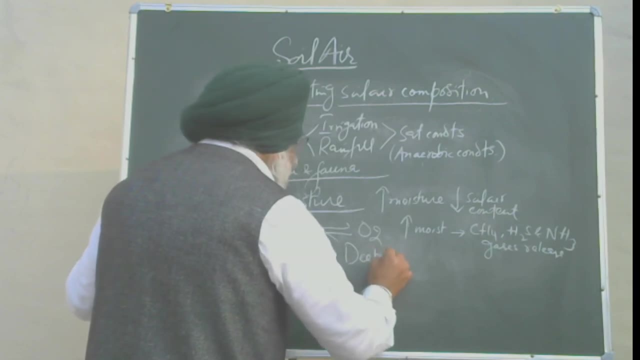 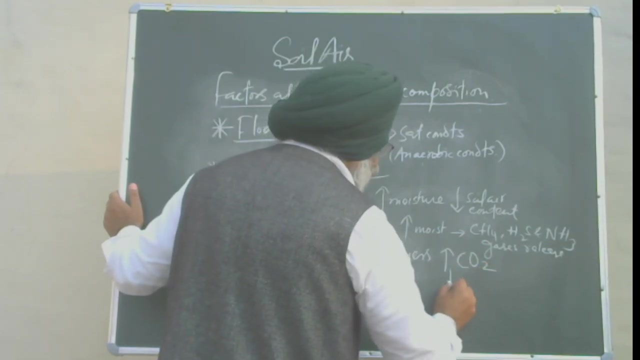 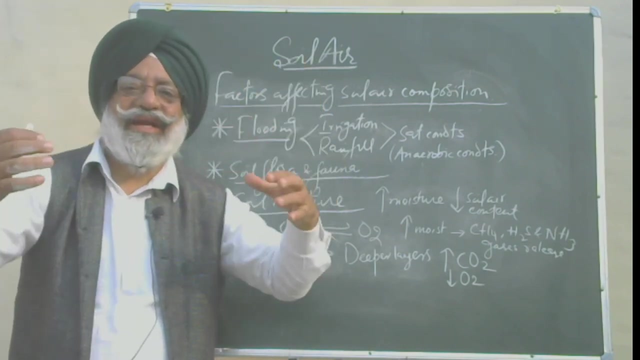 Because the composition of soil, here, you know it, is very much a function of the depth of the soil. So, first of all, as you go deep, the deeper layers should have higher carbon dioxide content and lower oxygen content. Why? It is because that in the surface layers, you know, have, you know, easy and higher. exchange of gases, maybe carbon dioxide, oxygen from the soil between the soil and the atmosphere, But this you know, exchange of gaseous or gaseous exchange. it decreases in the deeper layers. So then we should expect the deeper layers to have higher carbon dioxide and lower oxygen. 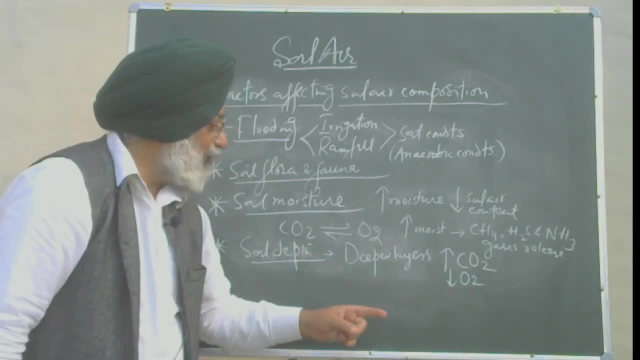 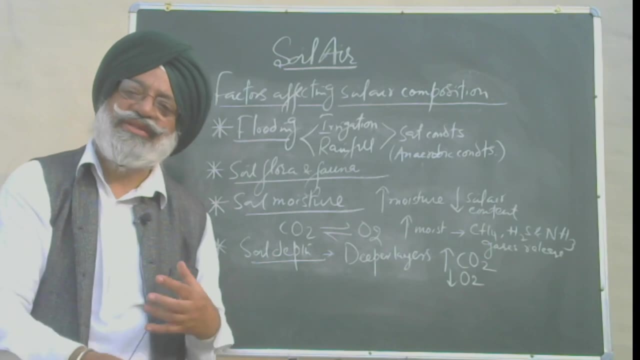 content And at the same time it is also because of the moisture content, Because as you go deep, the microprostate, even in medium texture, coarse texture soil, that microprostate also decreases, increases, sorry, and macroprostate decreases. 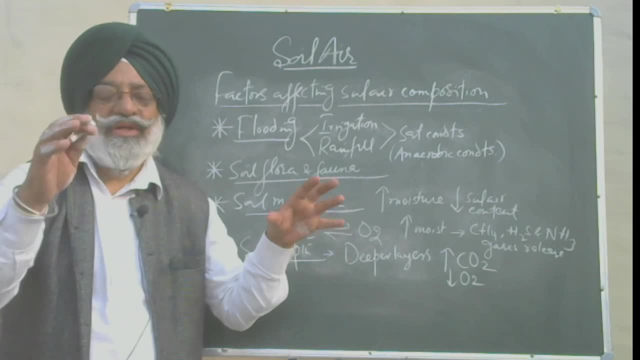 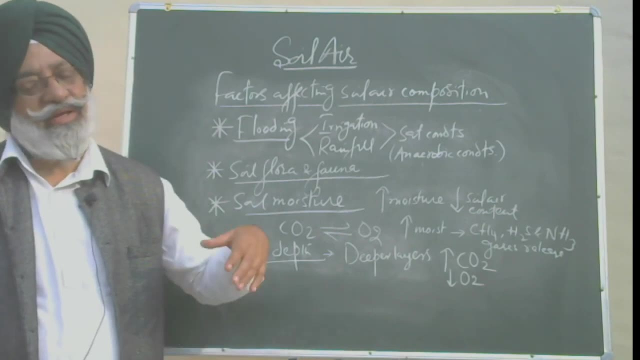 And you know macroprostate. they contain generally the air. So when you have a higher proportion of micropores in the soil, you expect the moisture to be higher, And if moisture is higher then of course carbon dioxide content will be higher. 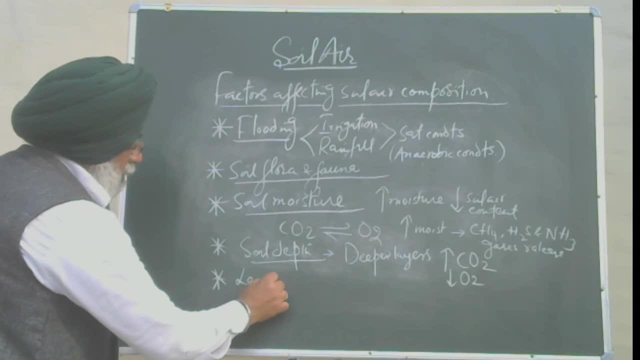 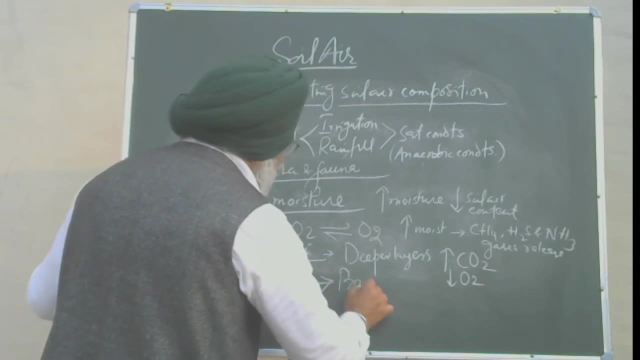 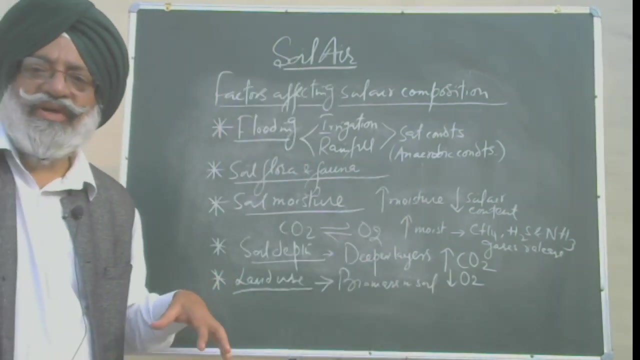 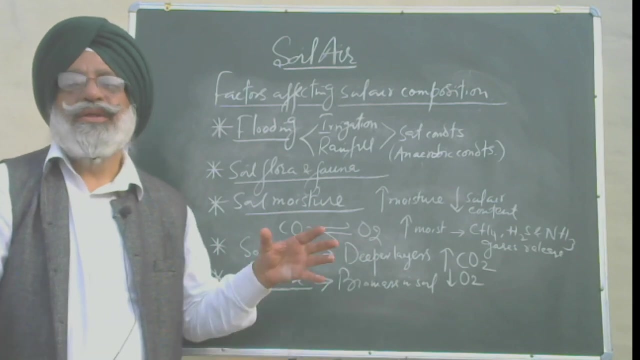 Then land use is another factor, Because land use will directly determine the biomass in soil. For example, if you have agriculture or cultivated lands, so in that case you can expect the plant biomass to be lower than grassland soils. So in grassland soils, particularly in the semi-tropical homes, well, if you cover for consultants a lot. but if you look at soil terms, the soilcamping of bio�uri combination, certainly the soil, if you look at everything and then you have healthy soil and then you have an üzerwater soil by right, desert soil, whatever you can call it, the underwater soil. 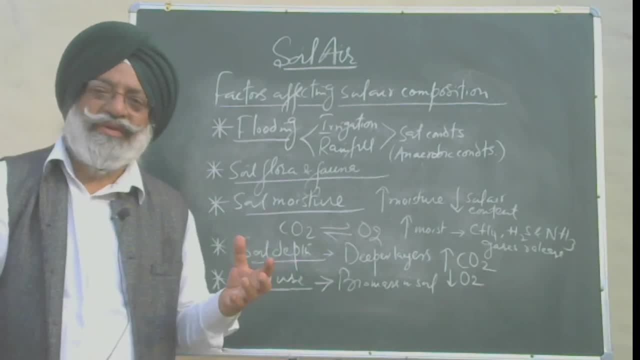 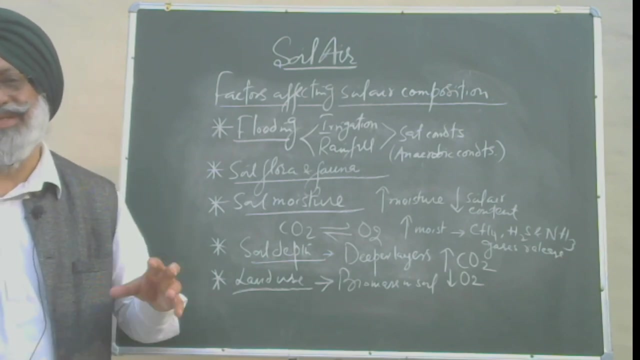 you gotta be aware of this. So, Thanks, surface layers. the microbial activity will always be here, because in grasslands there's a dense root system and roots continuously, they die and they become part of the organic matter and that's why in grasslands you have a very good, you know- soil structure. we have crumb type of structure. 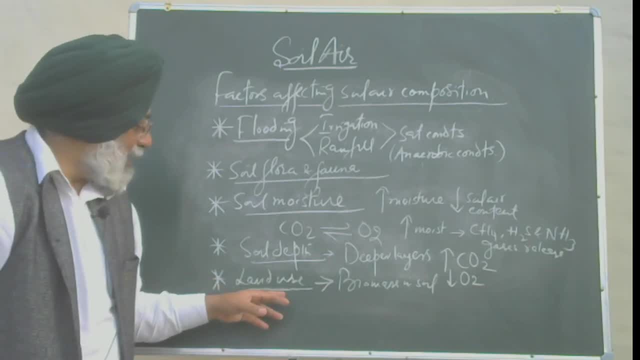 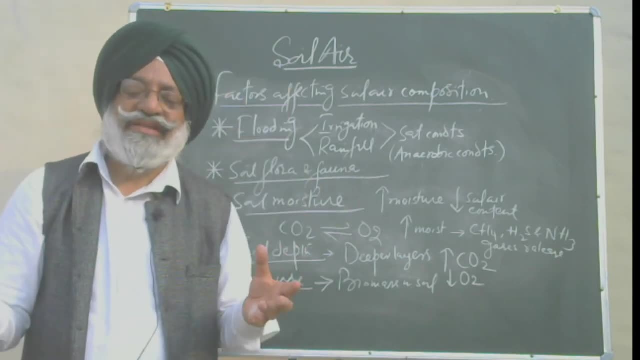 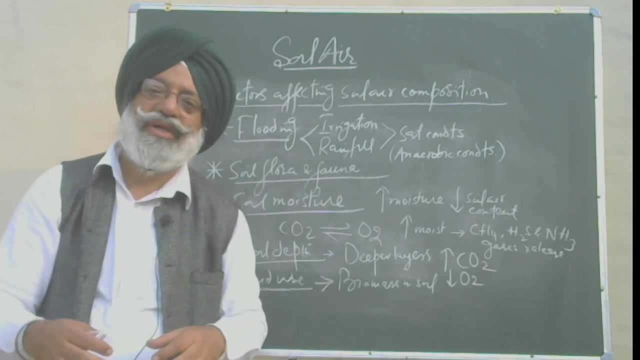 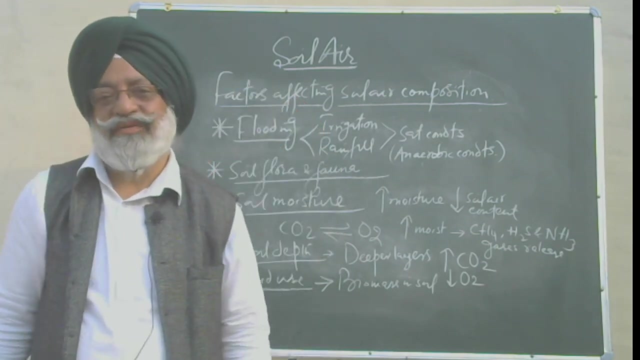 present in the surface layers and secondly, similarly, in forest lands or horticulture, where you have tree plants, trees, so a lot of litter remains continuously falling over the soil surface, ultimately becoming part of the soil. and if you till that particular soil, disturb the soil, that may go into the soil and microbial activities increase. so land use has a lot so. 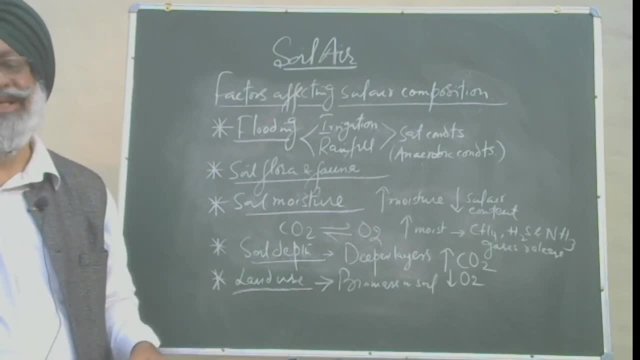 generally it has been seen that the soil organic carbon content in forest soils, in horticultural soils, is always higher. grassland soils is also very high- high in the surface layers- compared to that in the cultivated lands. so land use and higher organic matter content means higher microbial activity, and higher microbial activity means higher carbon. 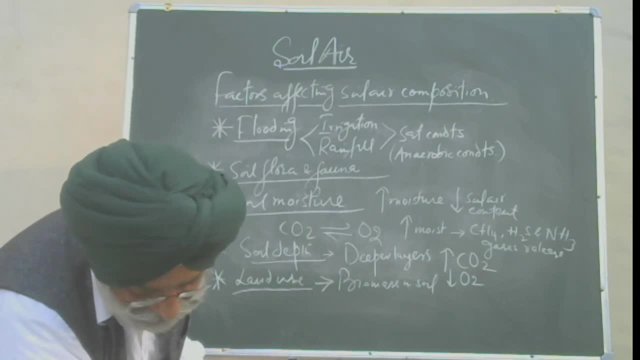 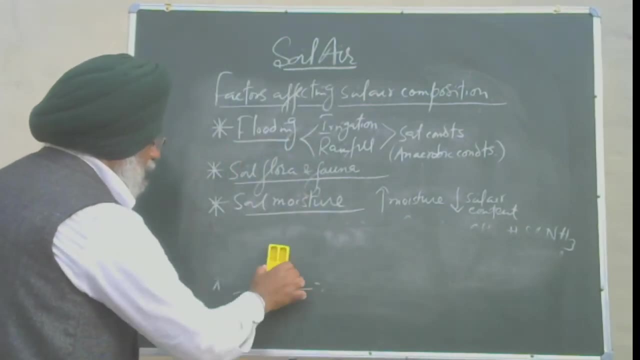 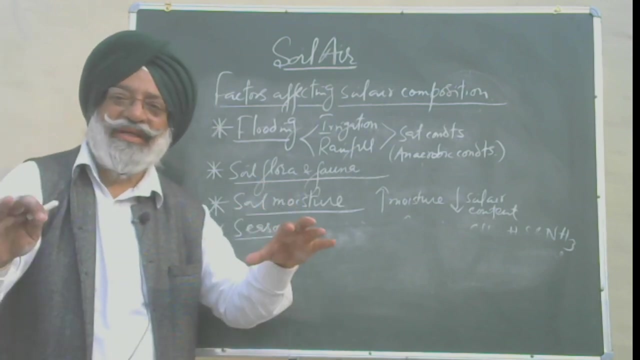 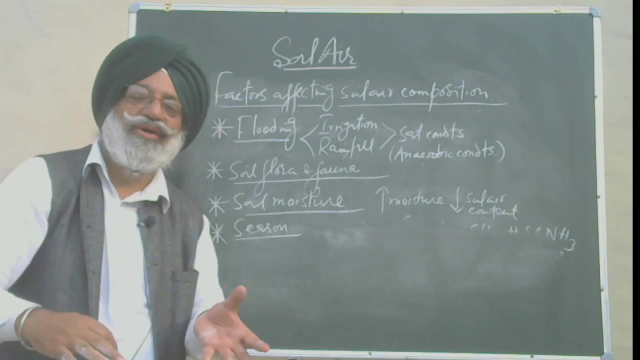 dioxide and lower oxygen content. so i hope the things are clear. then season is another important factor, and season, because season is also- ultimately it influences the microbial activity. if you have very low temperatures, winter season, the microbial activity subsides, it becomes less. but on the other hand, if you have the season where temperatures are high, moisture content is higher, then microbial activity will be higher. so basically will affect the microbial activity, which will be higher during summers than winters. and again, higher microbial activity means, of course, higher amount of carbon dioxide, lower amount of oxygen present in the soil. Then it also depends upon the cultural practices. This 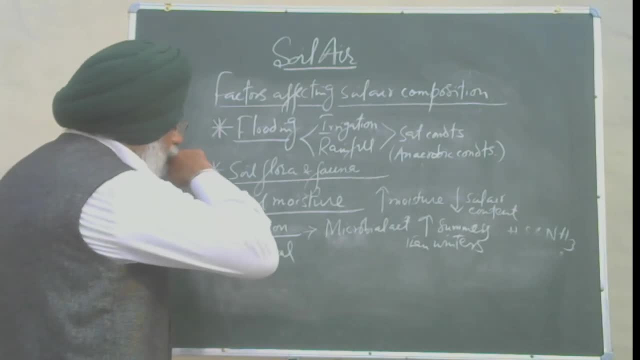 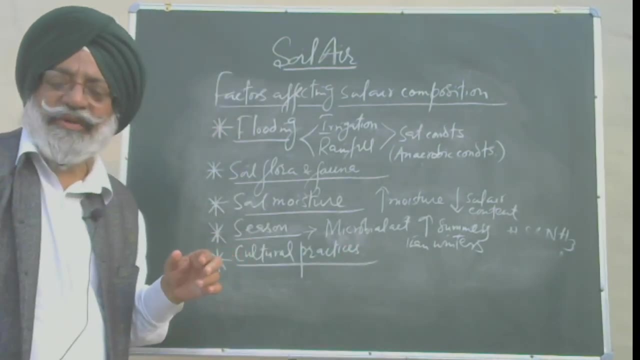 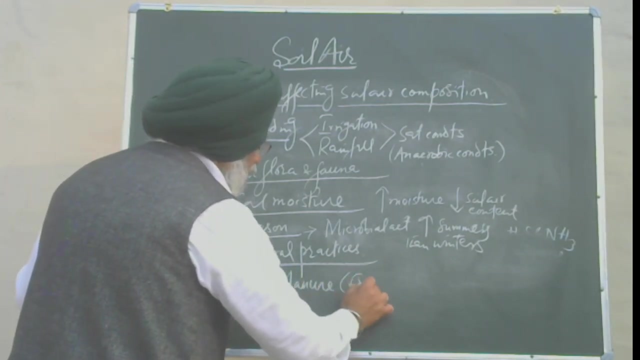 is again very important. So many factors are there which influence the composition of soil. As far as cultural practices are concerned, it could be manuring. If you are adding manures into the soil, it could be farm yard manure. it could be green manure, So that means you. 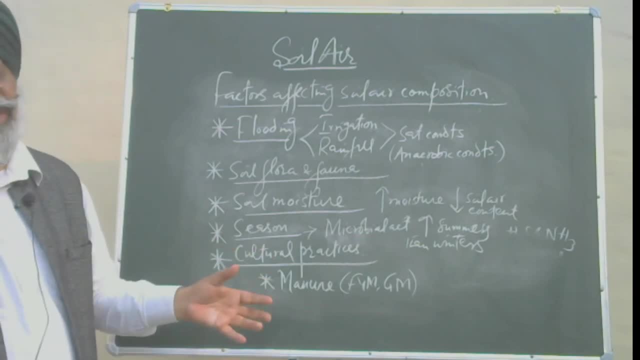 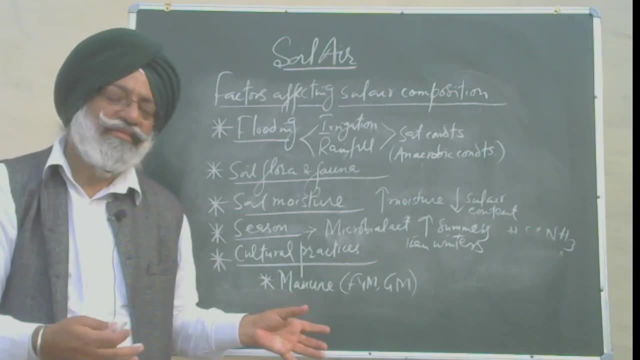 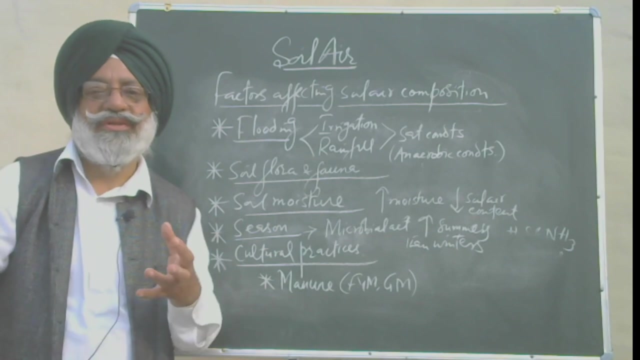 are basically adding organic matter into the soil, and when you add organic matter into the soil, you should expect microbial activity to be higher And at the same time, if microbial activity will be higher, carbon dioxide content will increase. So you have to keep a balance that how much organic matter or manures you have. 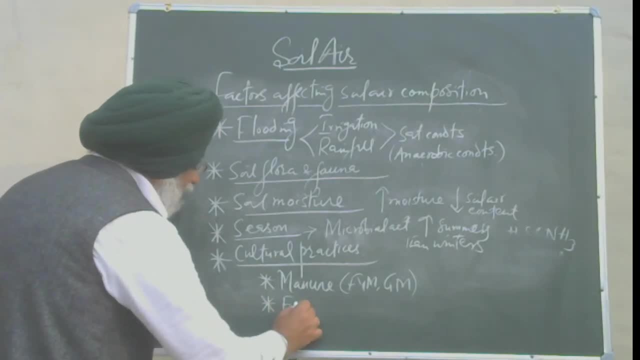 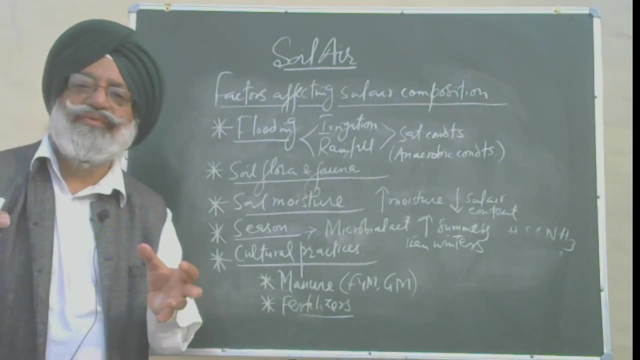 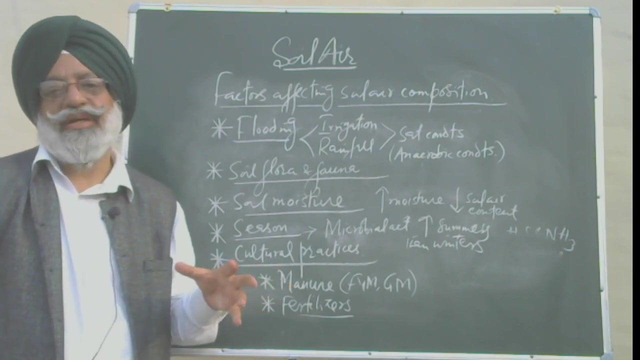 to add into the soil. Similarly, fertilization: When you add fertilizers into the soil, as I said, the conversion of nitrogen from imide form, the monocle form, to nitrate form. that is again accomplished by carbon dioxide, Different microbes, nitrifying bacteria, ammonifying bacteria, and their activity increases when. 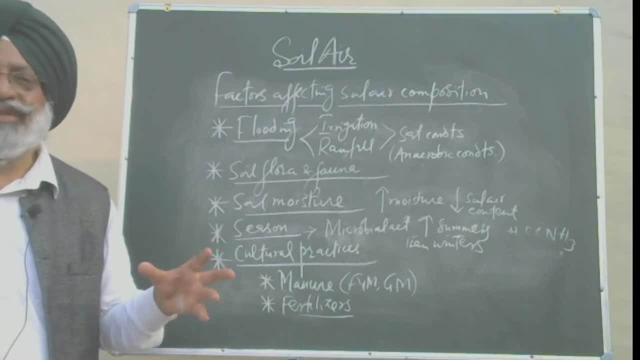 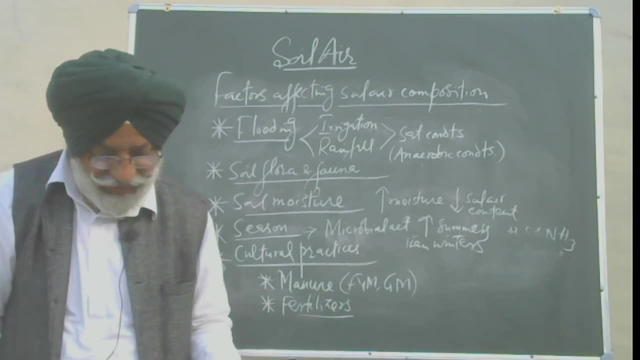 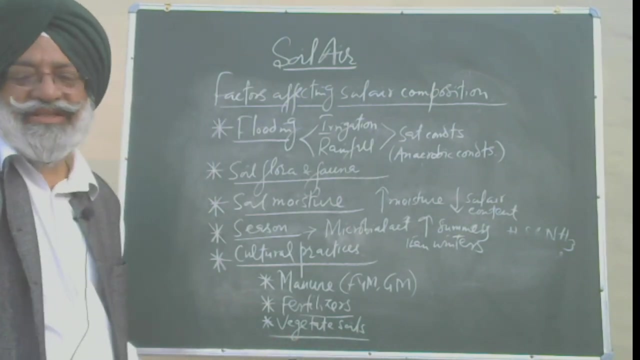 you add fertilizers into the soil, And particularly when the temperatures are optimum, when sufficient moisture is there, so microbial activity will be higher and carbon dioxide concentration will go up. Similarly, in vegetated soils That means when vegetation is there, then as compared to bare soil, In bare soil you don't expect much. 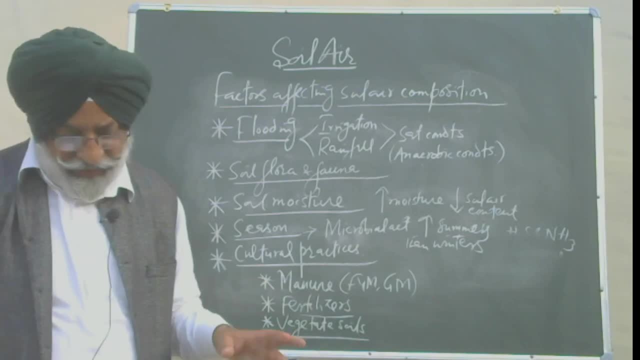 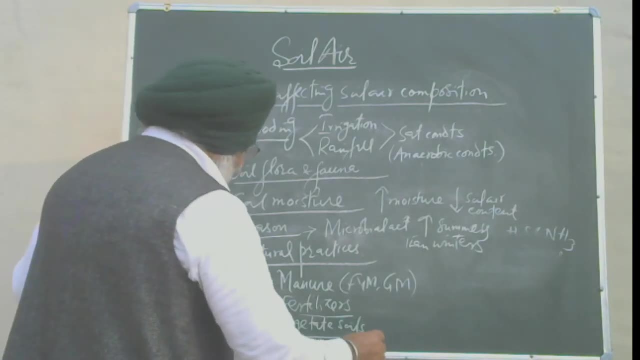 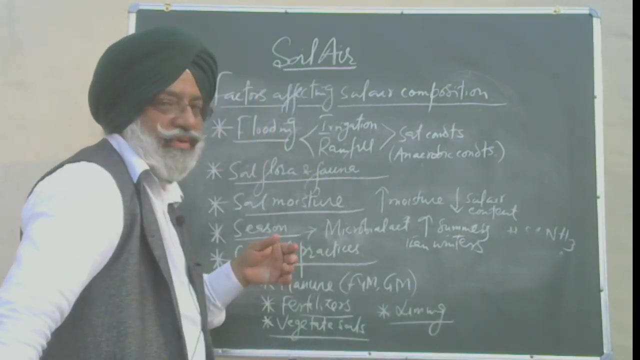 microbial activity as compared to vegetated fields. So again, the microbial activity that will increase in vegetated fields. Then liming also. When you add lime, the liming also creates favorable conditions for higher microbial activity. So most of these factors, whether 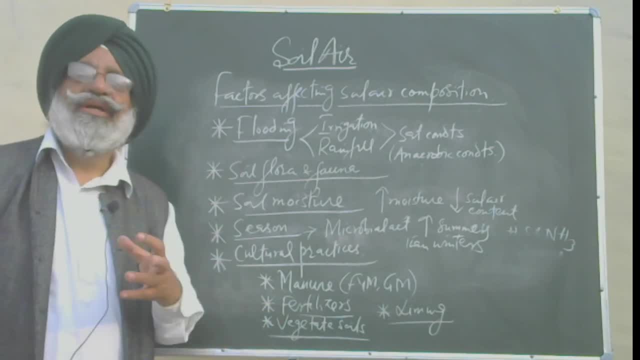 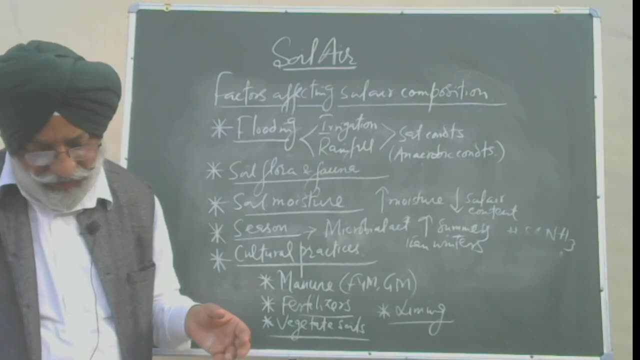 these are flora, fauna. all these are favorable and favorable conditions for higher microbial activity, moisture season culture practices. they ultimately they affect, you know, the microbe activity in the soil and that determines the amount of carbon dioxide and oxygen present in the soil. so, in nutshell, the chemical activities. 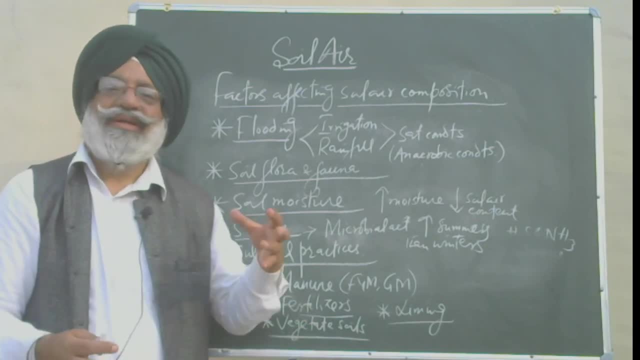 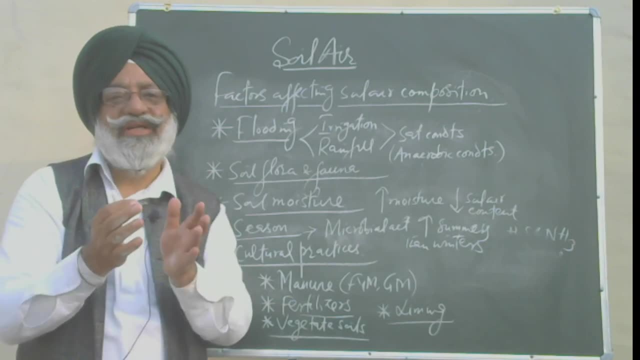 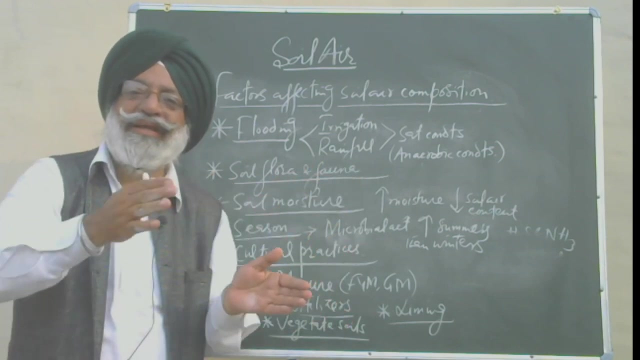 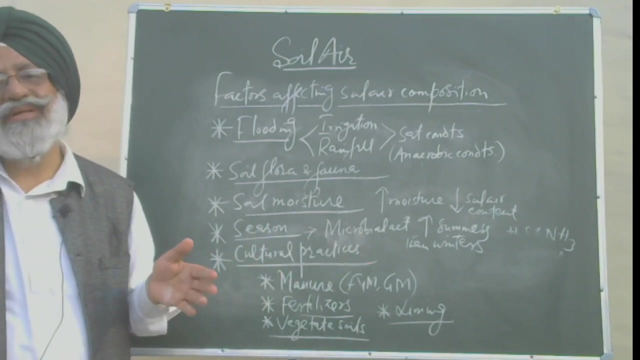 biological activities in the soil. they affect the composition and they, when you have higher chemical activities, are political activities. so that means the gap between the composition of soil here and atmospheric air that is accentuated, it increases. but on the other hand if you have some physical you 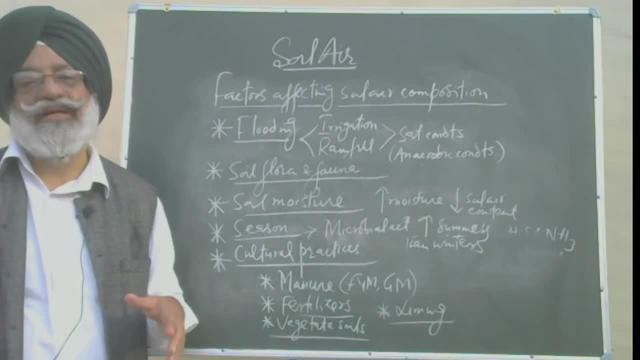 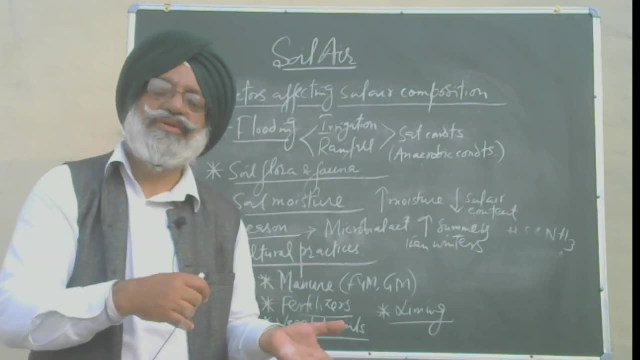 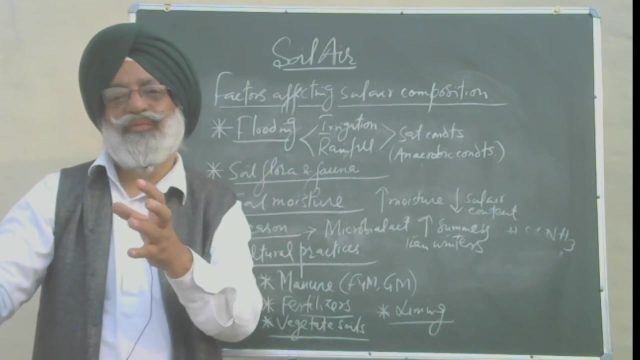 know processes, physical characteristics like your, macro porosity, micro porosity, texture of the soil, structure it because texture and structure of the soil they ultimately determine macro porosity and micro porosity. so there should be an ideal balance. of course you should have 50% of micropores, 50% of macropores. only then you can expect. but